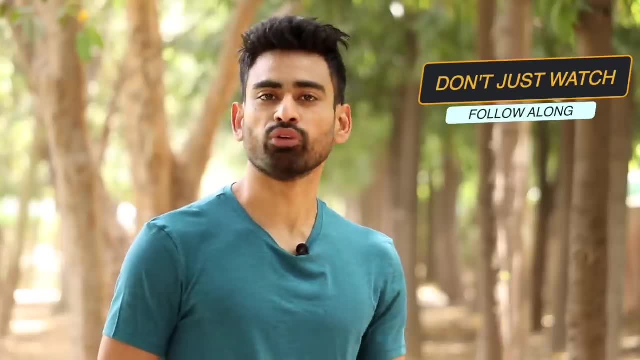 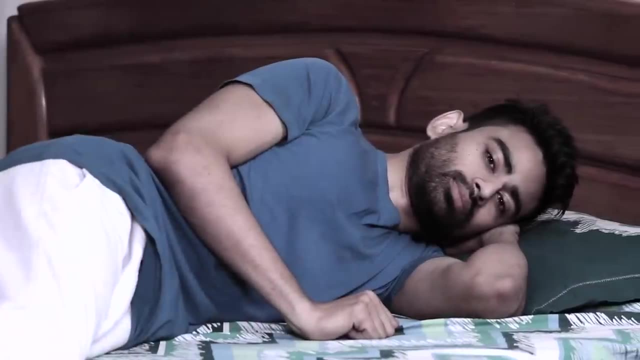 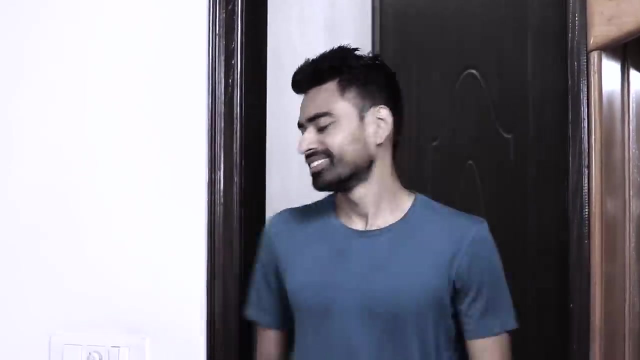 video. One more thing: this video is not just to watch, but to follow along. So come on, let's do it together. Hello friends, welcome to Fit Tuba. Every morning, after waking up, drink water, freshen up and get ready to practice yoga, preferably outdoors, without eating anything. All you. 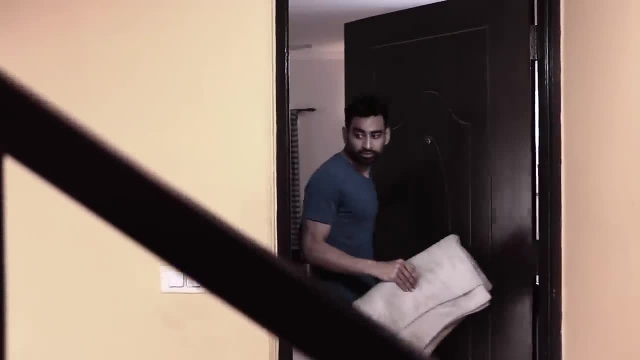 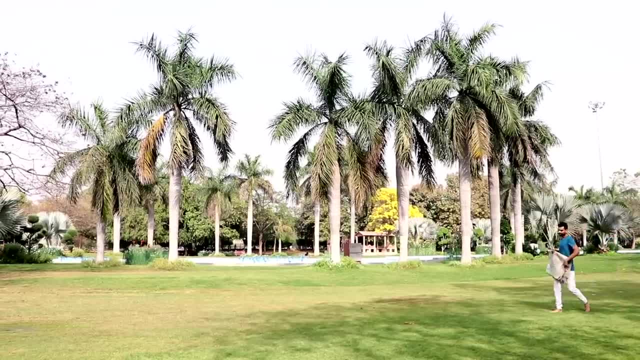 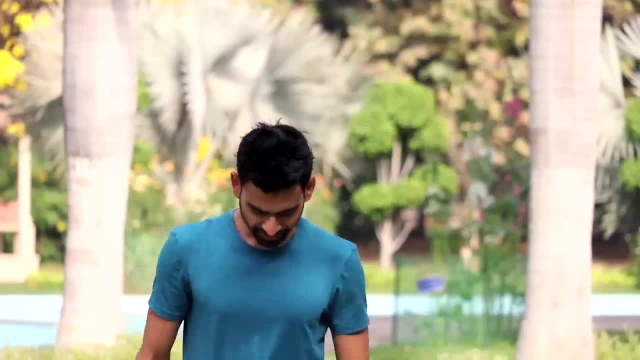 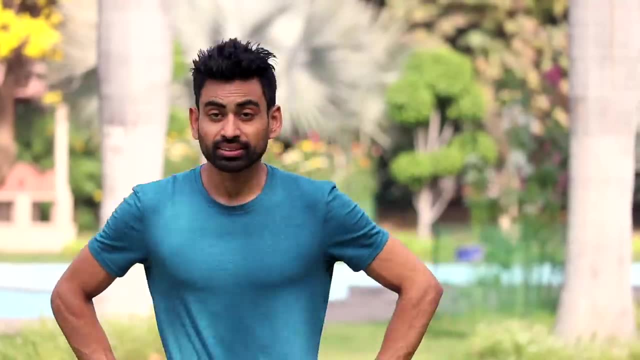 preferably made of cotton, wool, or you can even use a towel or a bed sheet. it is important to prevent the earthing of the energy that will get generated in your body. the effectiveness of doing yoga multiplies when we begin by proper lubrication of the joints, so let's do that with a quick warm-up. 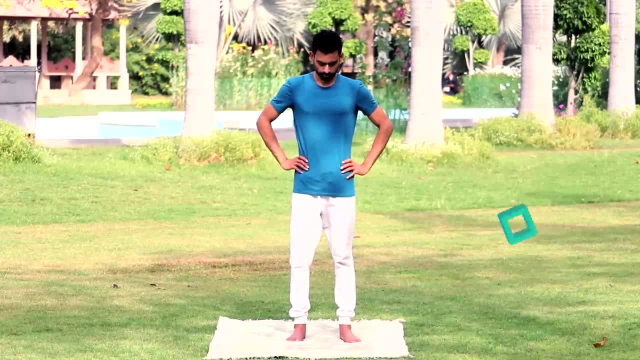 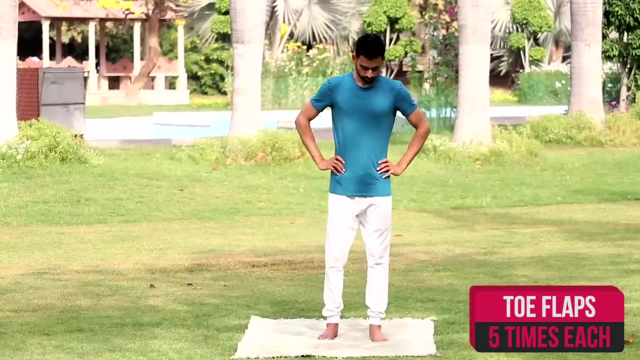 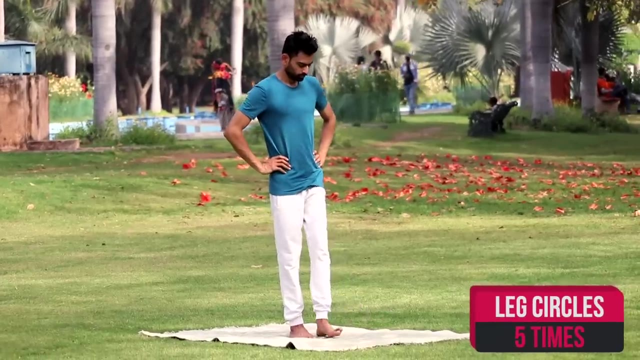 rhythmically moving up from toe to head. stand straight, facing the east direction, starting with the left toe. move it up and down five times. now lift the right toe and in the same way, move it up and down for five times. moving up, lift your left leg a. 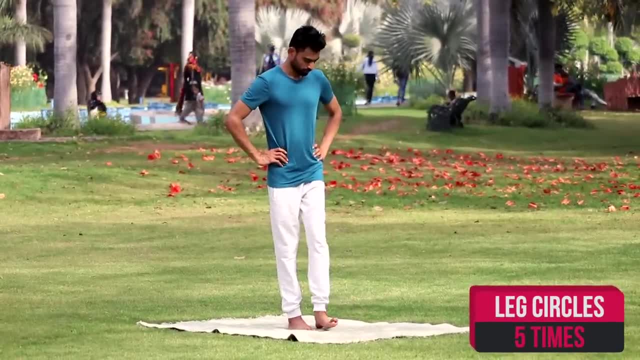 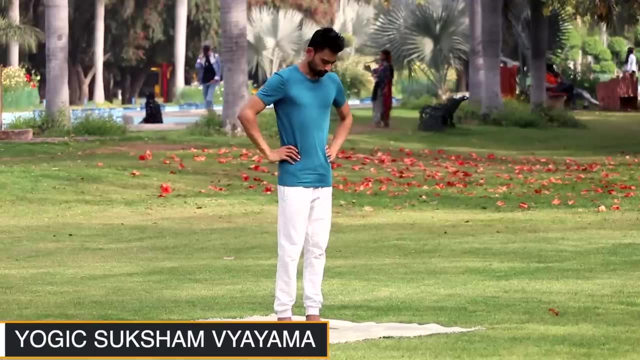 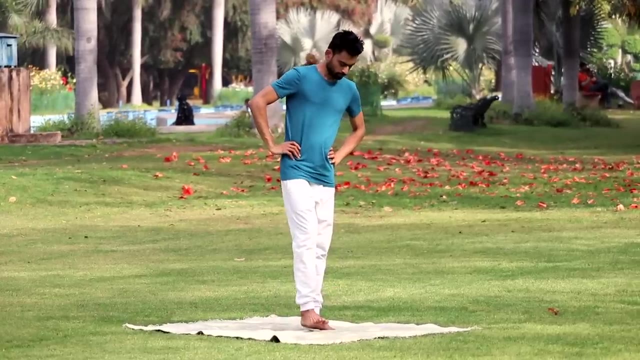 bit and rotate it five times in clockwise direction and then five times in anti-clockwise direction. these micro exercises are called yogic sukshma vayam. now, similarly, lift the right leg and rotate it five times in clockwise direction and then five times in anti-clockwise direction. 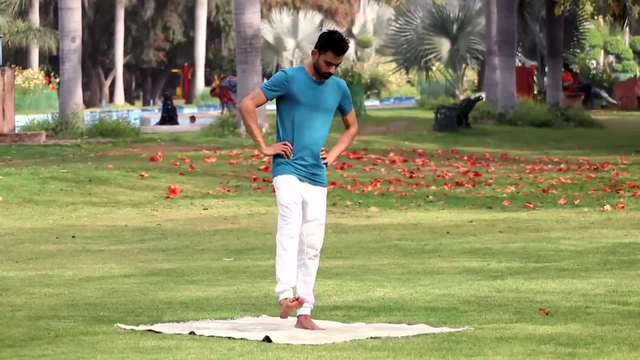 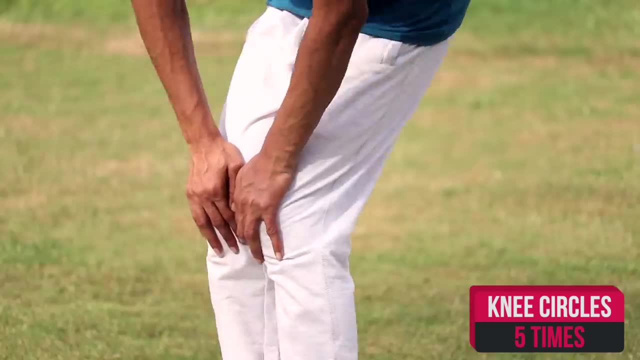 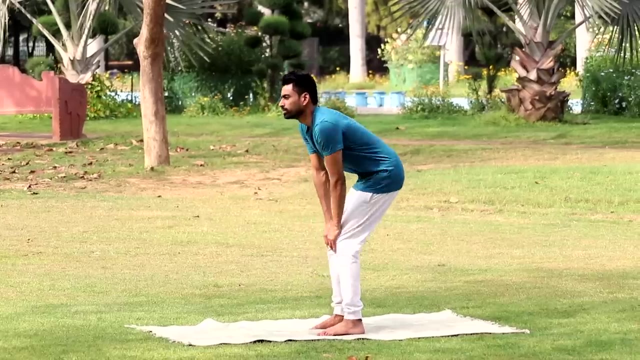 yoga is all about doing comfortably at your own pace. Yoga is all about doing comfortably at your own pace, with a positive state of mind. now bend your knees, place your palms on it and then rotate them clockwise, and then anti-clockwise, five times each. these seemingly minor exercises are powerful. 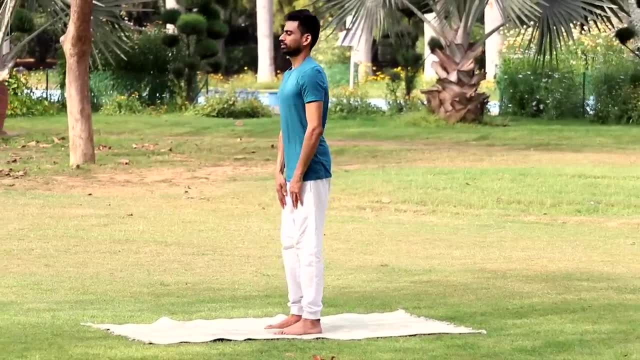 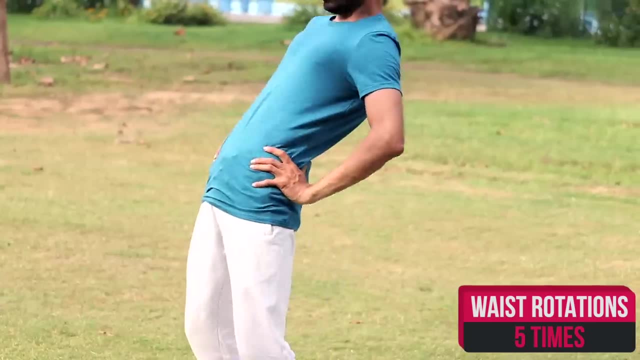 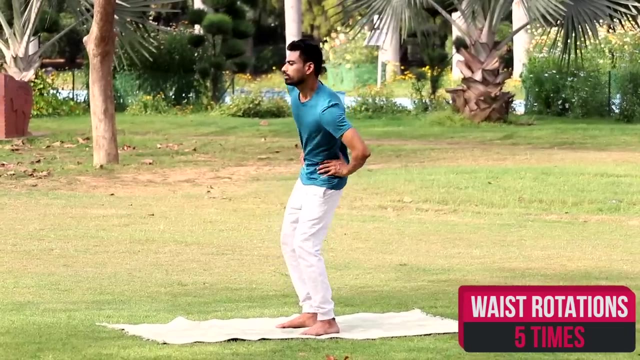 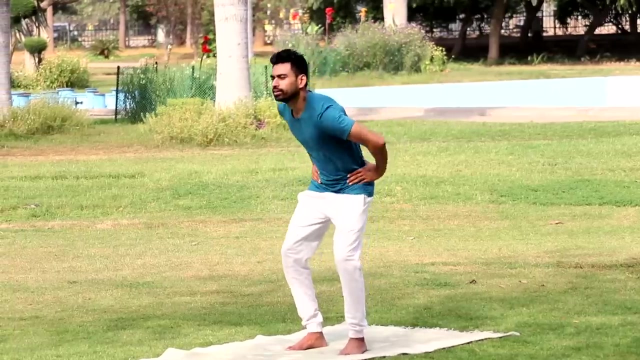 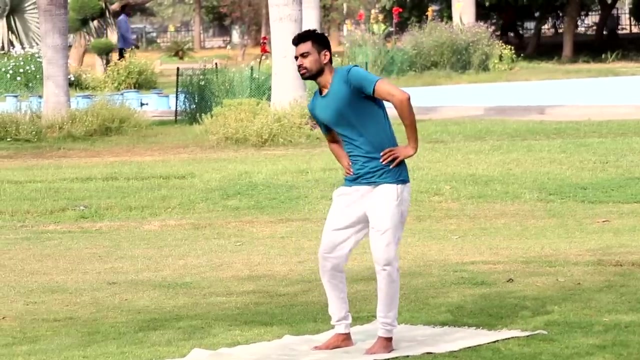 as they activate the subtle channels of the body. now place your hands on the waist and rotate it five times clockwise and then five times in an anti-clockwise direction, if you want to start. gaiters and homeostasis are powerful quite often. let's see how. let's see how we can Capricorn. 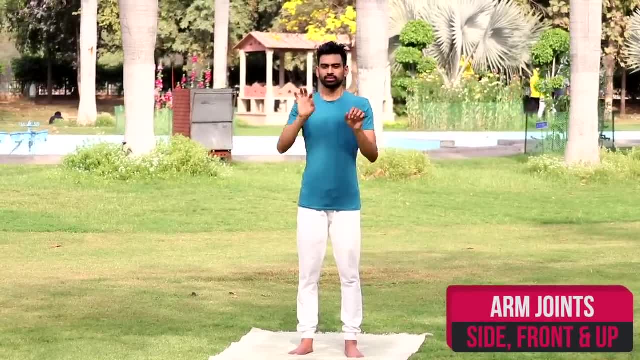 end, vibe, sit down and sit still and please cross your legs from side to side to side and sit. need~~ finish and finish and do this exercise three times per day. total men: ten minutes and two break in. I always feel exhausted because at this state, ten minutes. 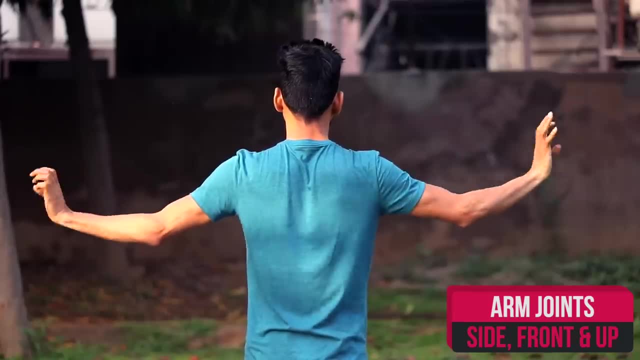 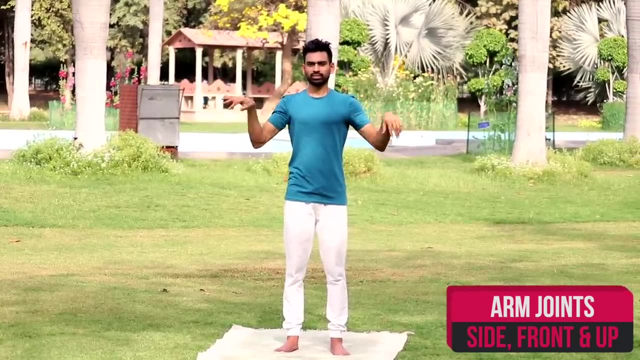 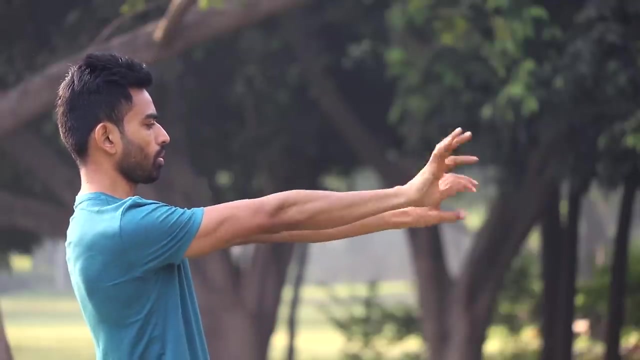 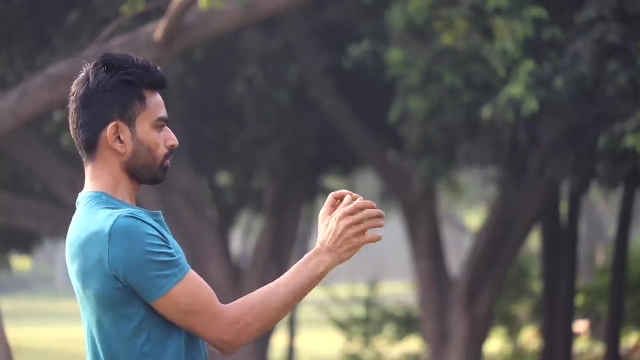 time is my favourite part of the body's functioning and it causes me switching. idiot because Chepstin's Rest sideways and then clench and relax 3 times. Go back and this time bring them forward. This exercise will tone your arms, making the wrists stronger and gripping power better. 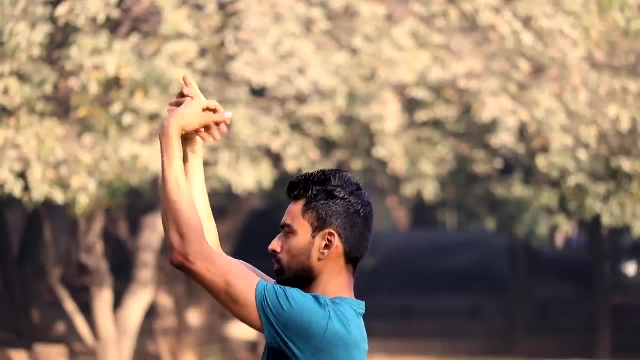 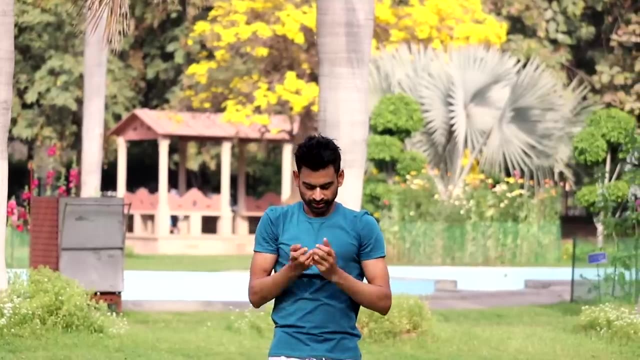 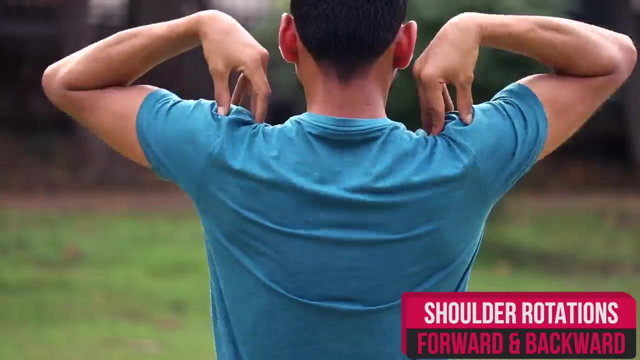 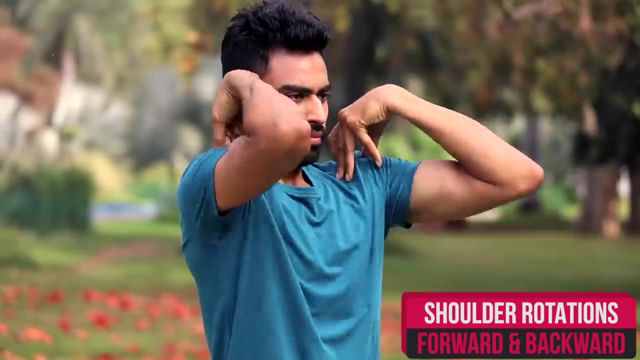 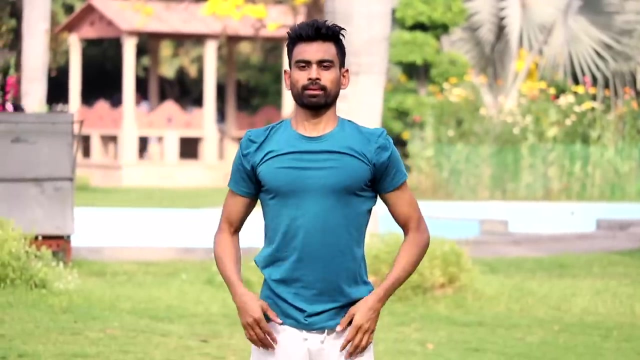 This time go up, Do it with complete involvement and a smile on your face. Now place your fingers on the shoulders like this and rotate them forward and then backward, 5 times each. Do it slowly, making a circle, without straining yourself at any moment. 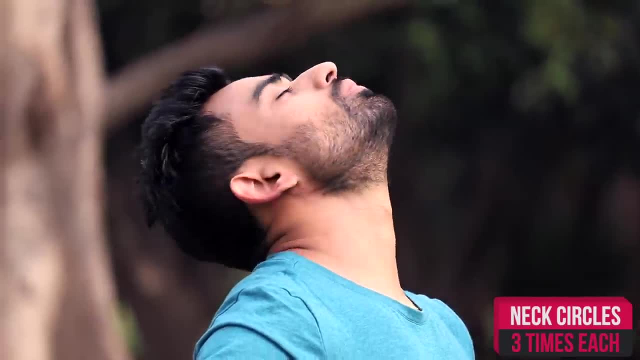 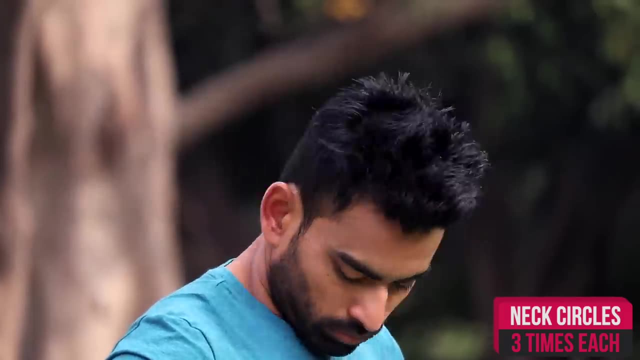 Now with your hands, place your fingers on the shoulders like this: Now place your hands on your waist. rotate your neck 3 times, first in clockwise direction and then 3 times in anticlockwise direction. Do it at your own pace, rotating it properly. 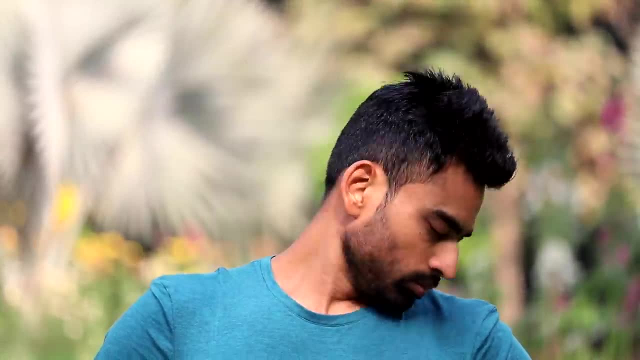 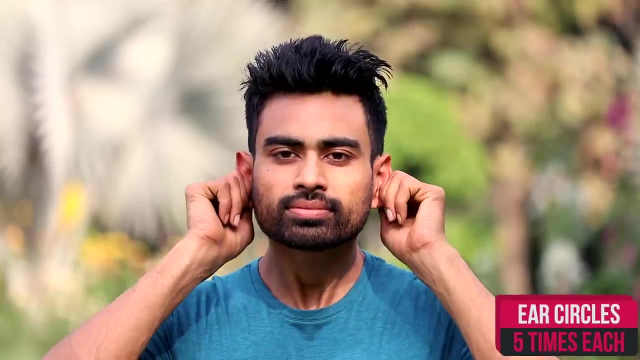 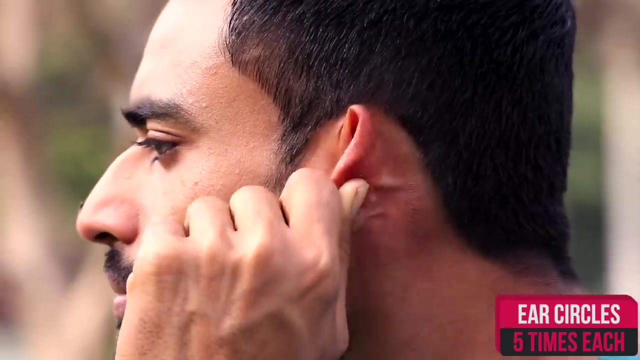 Feel the tension getting released of your neck muscles- very effective in preventing cervical problems. Now hold your ears and move them, clockwise and anticlockwise. Do this 5 times each. The nerves that increase. pragya ie: awareness is located in our ears. 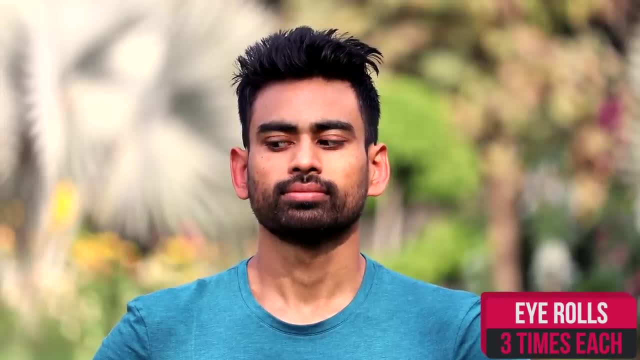 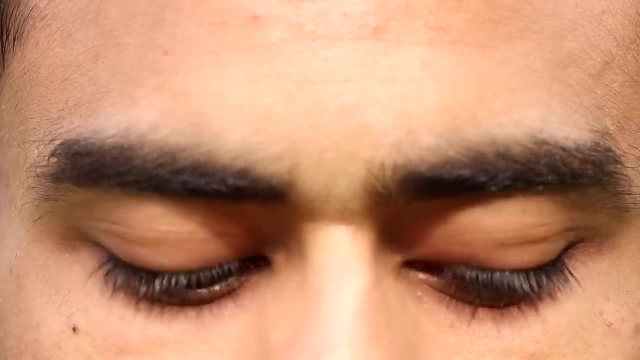 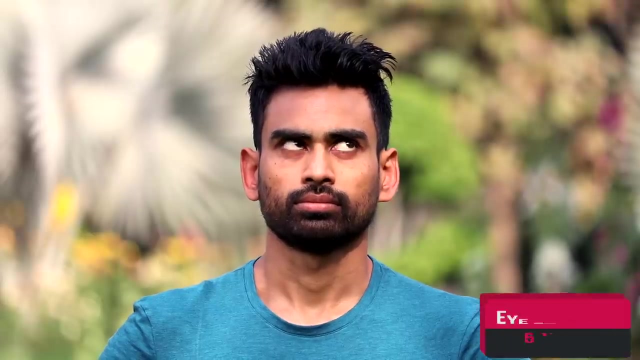 Moving to eyes, Roll your eyes clockwise 3 times and then 3 times in anticlockwise direction. Now, roll your eyes clockwise 3 times and then 3 times in anticlockwise direction. Roll your eyes clockwise 3 times and then 3 times in anticlockwise direction. 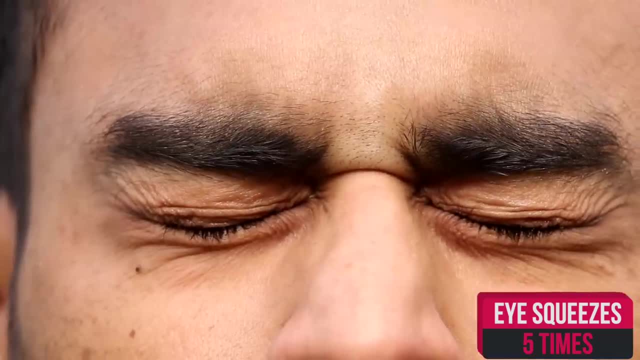 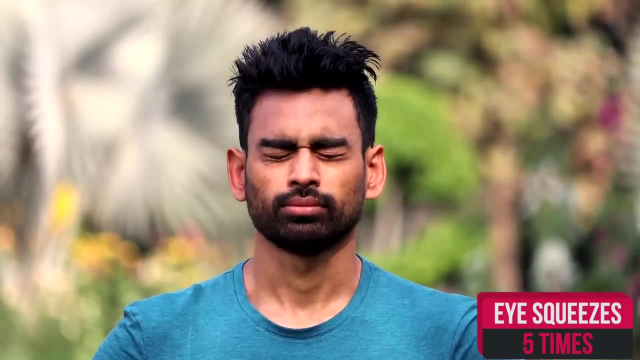 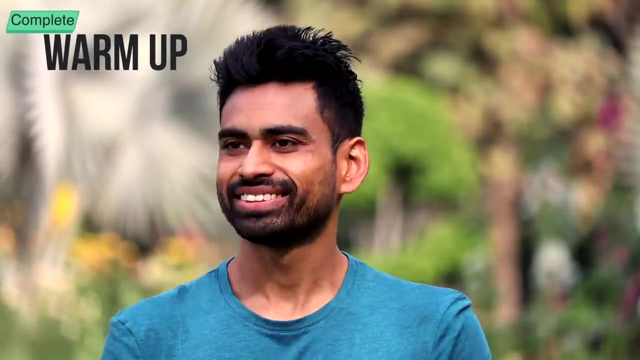 Now squeeze your eyes tight and place your fingers on the chest. Replace the hands, Do it with complete support and then open them wide 5 times. In this day and age, eye muscles definitely need a lot of exercise. So this completes the warm-up to increase the flow of pranic energy throughout the body. 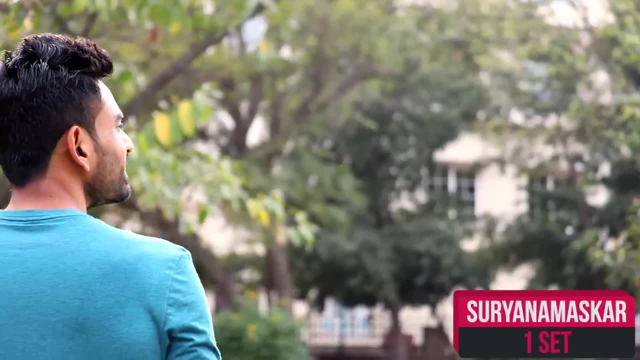 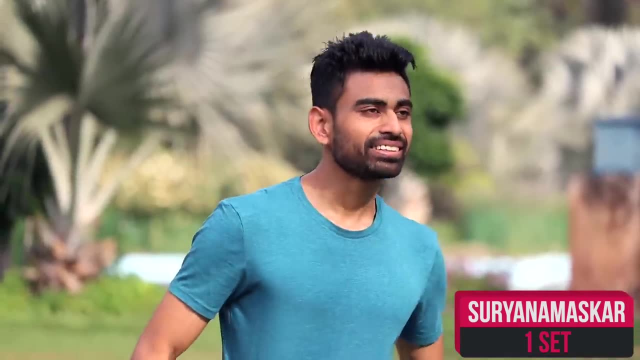 Well done. Now our body is ready to do. Surya Namaskar. It is a powerful Kriya to instill the sun's energy within you. Listen to it with a sense of gratitude to the sun for sustaining life on our planet. 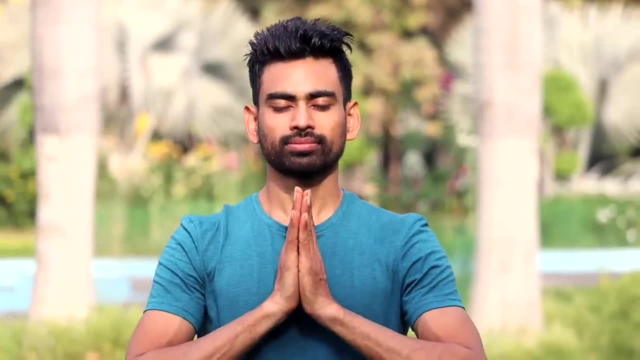 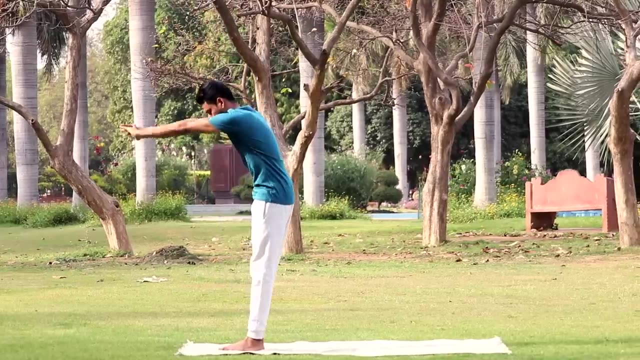 Facing the sun. come to the edge of the mat, Hold Anjali Mudra, Take a deep breath in and lift your arms up and back. Now breathing out, bend forward and bring the hands down to the mat beside the feet. Do it comfortably. 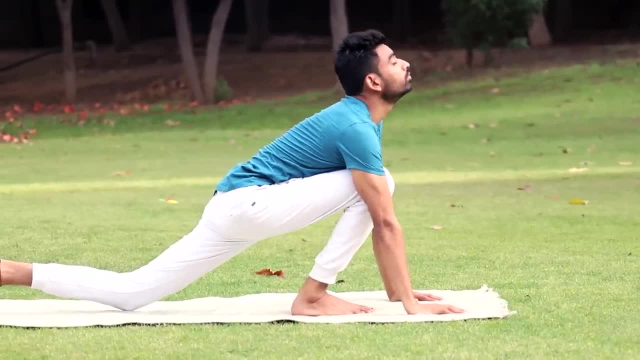 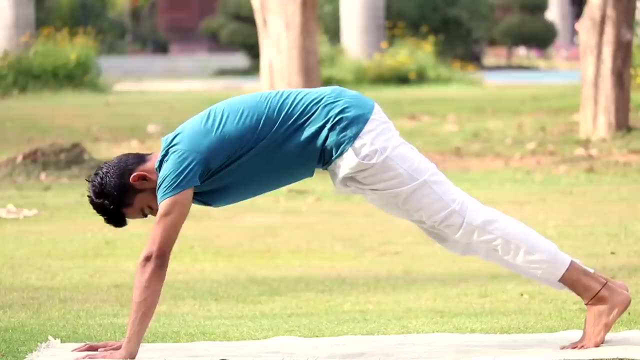 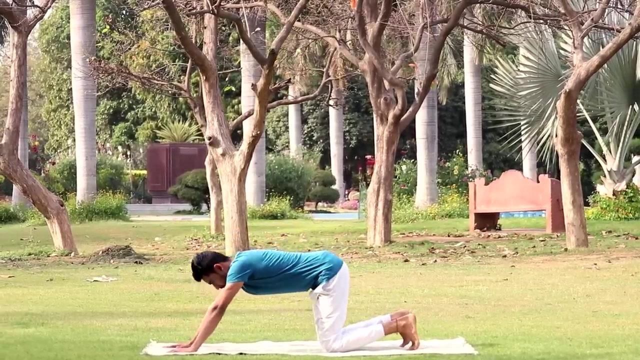 Now breathing in. push your left leg as back as possible, right knee being in the front. Look up Now. take back your right leg also. Move your back up with eyes on the navel. Now gently bring your knees down to the floor and exhale. 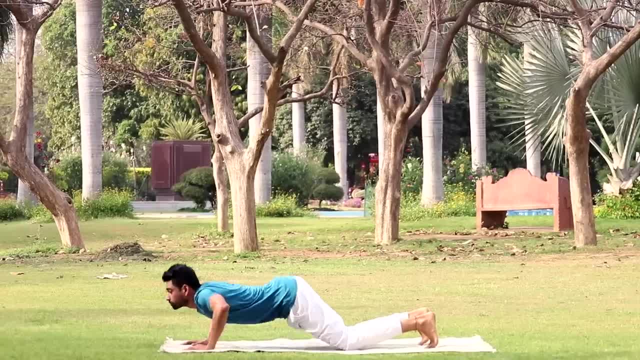 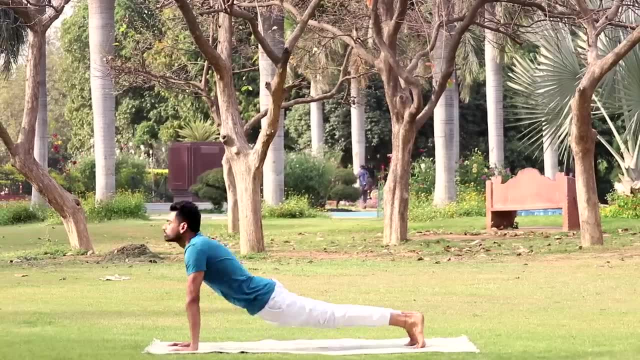 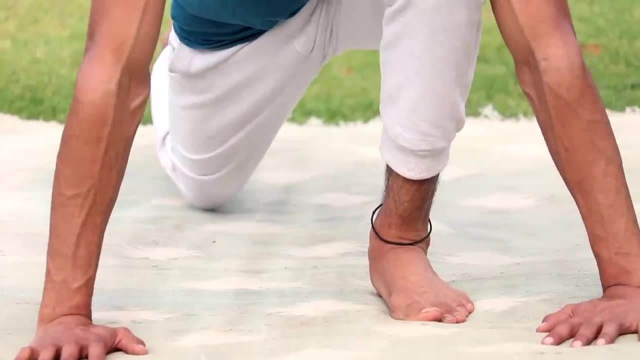 Rest your chest and chin on the floor, Then slide forward and raise your chest up into Cobra pose. Look up Now, breathing out. lift the hips to bring your body into an inverted V pose. Take a deep breath in And this time bring your left foot forward in between the two hands. 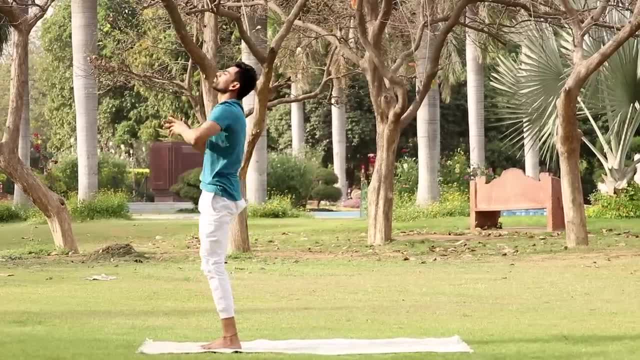 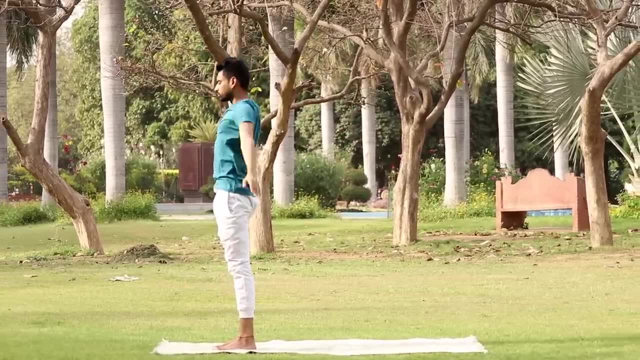 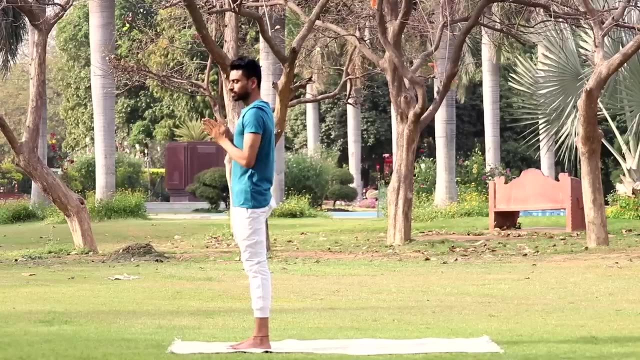 Breathing out. bring your right foot forward Now. stand up, Take a deep breath in, raise your hands up and bend backwards As you exhale. first straighten the body, then bring your arms down sideways. Relax. How do you feel? 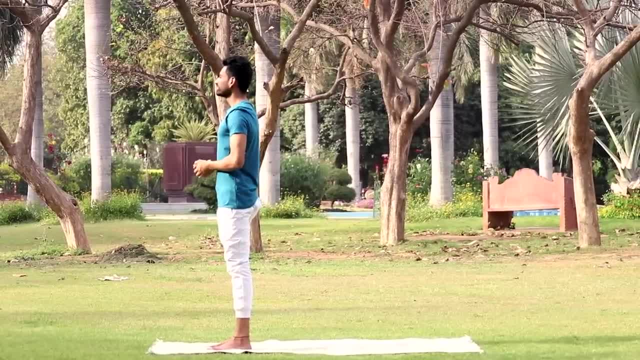 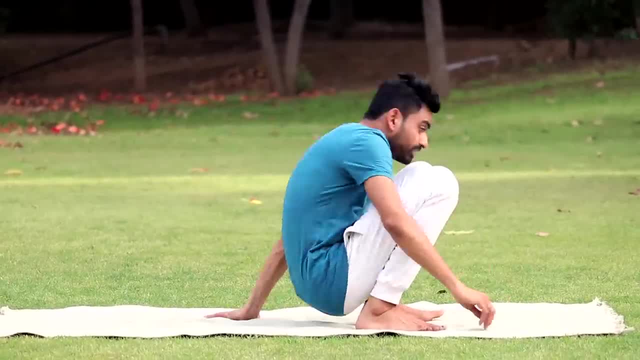 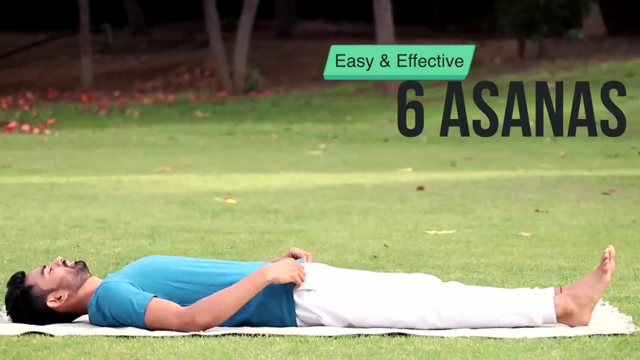 Not just on the body. Surya Namaskar is known to have an immense positive impact on the mind as well. Now lie down on the mat. Before moving on to the breathing exercises, we will practice six asanas which are relevant and effective in curing our modern-day health problems. 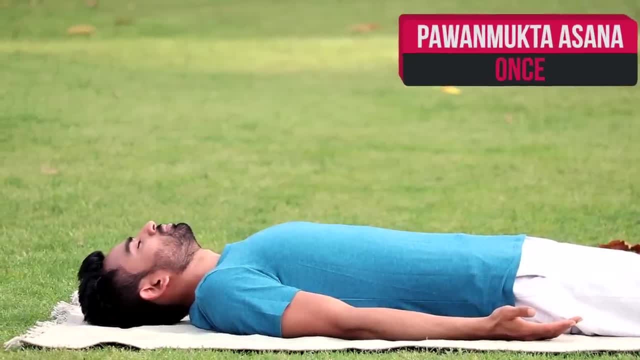 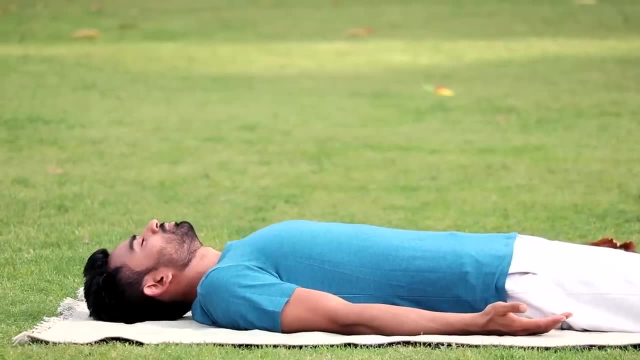 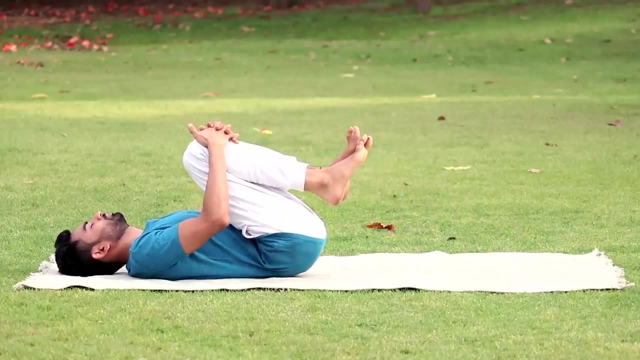 First is Wind Relieving Pose: the Pavanmokta Asana Arms beside the body, palms facing the ceiling legs together. breathe in and, as you exhale, bend both your knees and bring them towards your chest. Interlock your fingers, press your thighs on the abdomen, lift your head and chest off. 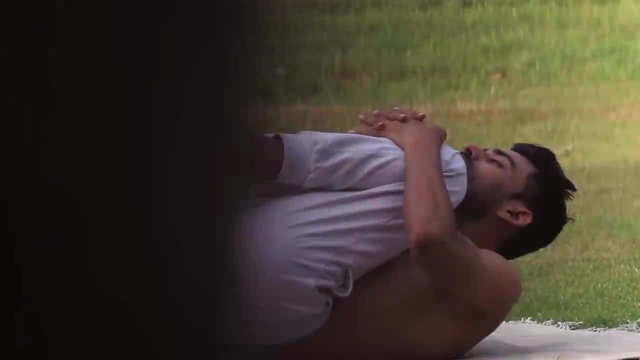 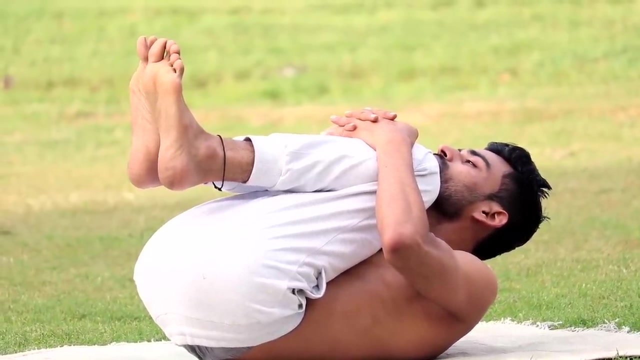 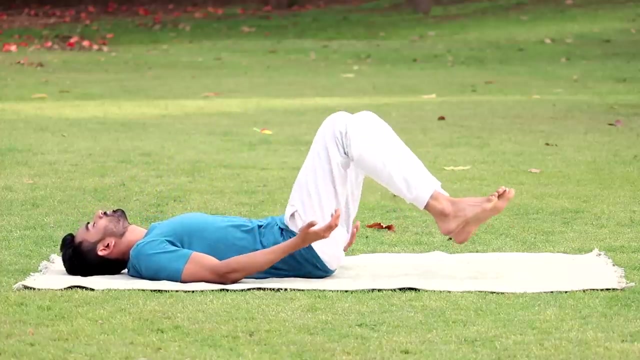 the floor, trying to touch your nose and then your chin. Hold this position for about 10 seconds. As its name suggests, Pavanmokta Asana massages the intestines, helping in digestion and release of abdominal gas. Now release your head, your hands and then your legs. 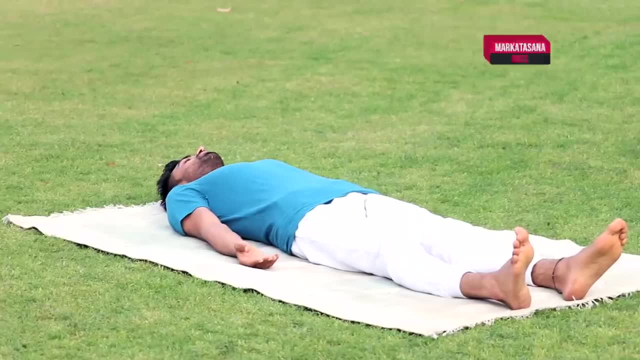 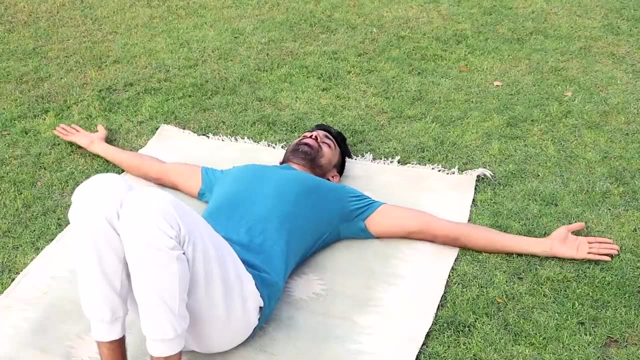 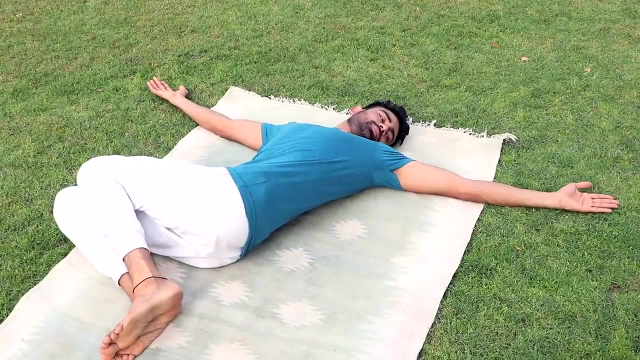 Relax. Next is Markat Asana, The Monkey Pose. Bend both your knees and keep them near to the hips. Spread both your arms at the level of your shoulders. Now turn both your knees together towards the right side, while your neck towards the. 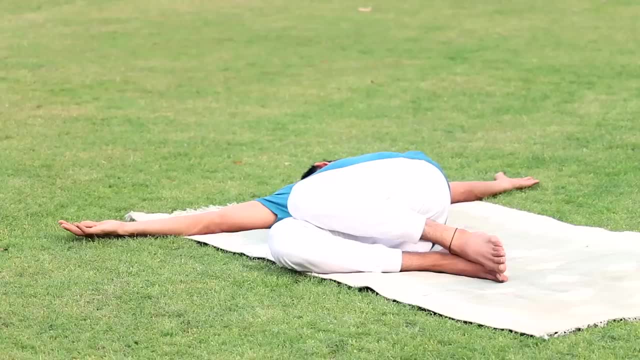 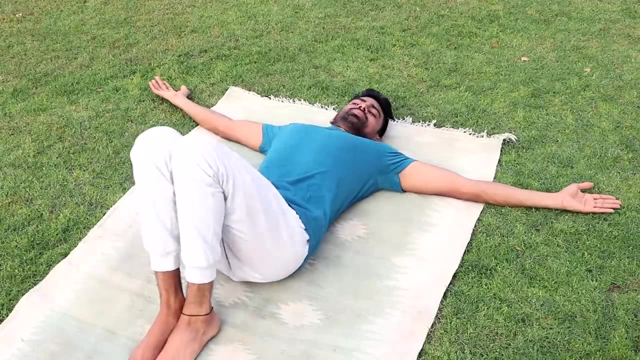 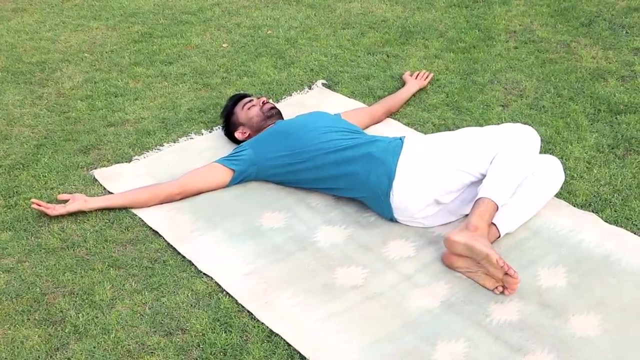 left side. Hold it there for a few seconds, Breathe normally as your spine is gently being stretched. Now slowly come back to the previous position. This time move your knees towards the ceiling, Keep your hands straight and keep your hands on your toes towards the left while your neck 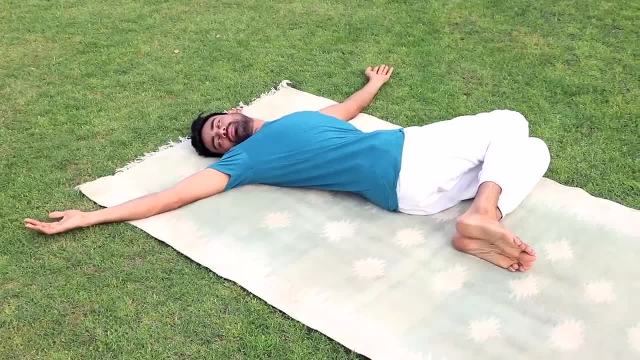 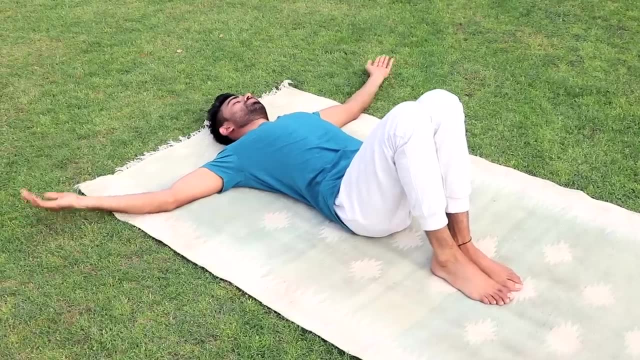 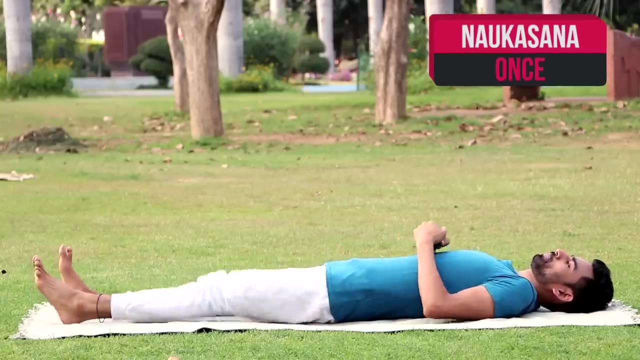 towards the right. Hold here for a few seconds. Markat Asana also promotes creativity, bringing our monkey mind to rest. Now come back to the previous position. Slowly stretch your knees down and relax, Moving on to the Nauka Asana, the Boat Pose. 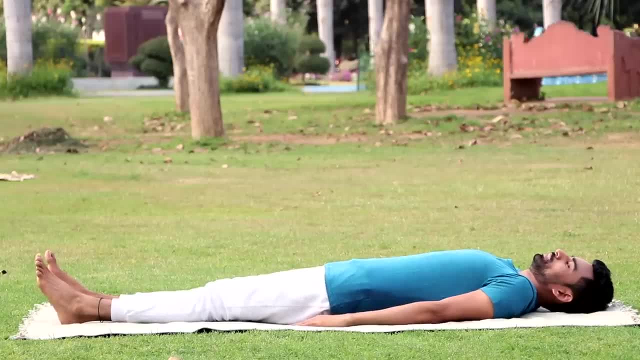 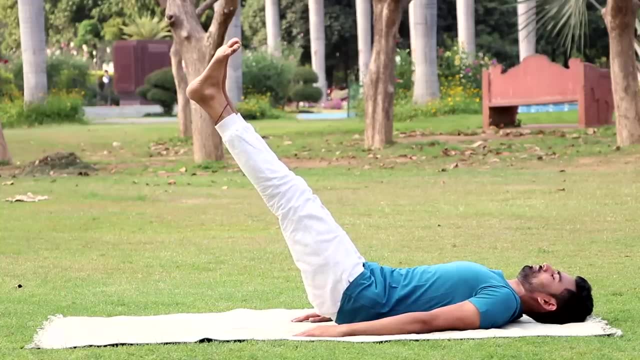 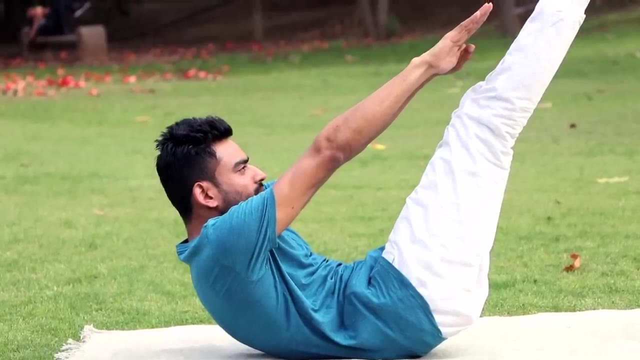 Keep your arms straight, fingers outstretched towards the toes, deep breath in and, as you exhale, lift your feet off the ground till about 45 degree angle is reached. now stretch your arms towards the feet. hold it there with your entire body weight on the buttocks. highly beneficial in reducing the extra. 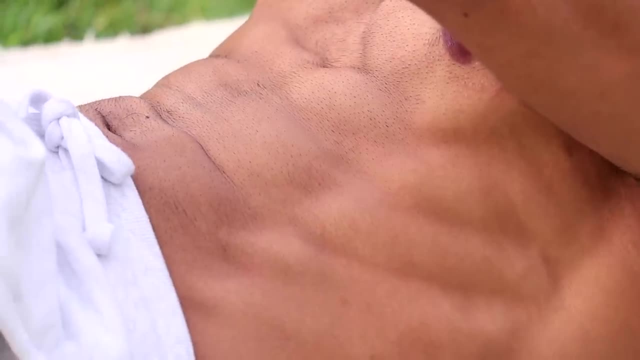 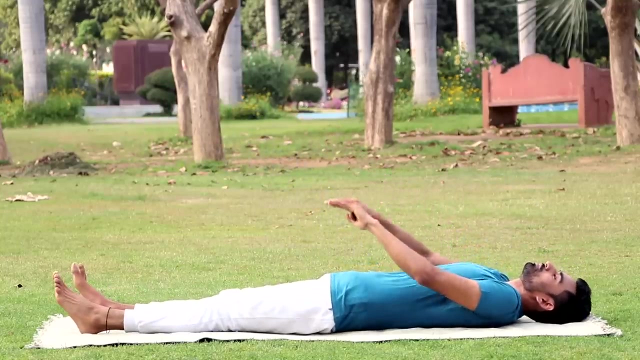 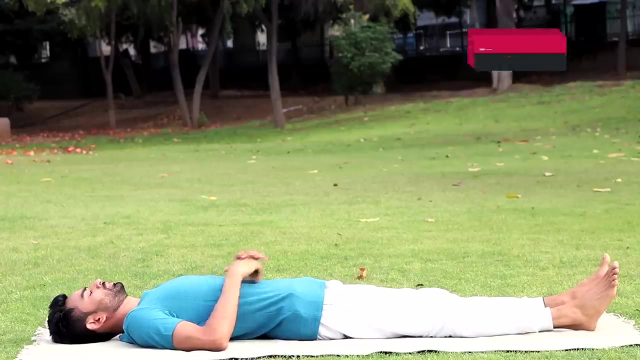 fat in the belly area. it strengthens the abdominal muscles. feel the tension originating in your ab muscles now exhale slowly as you bring the body to the starting position and relax, moving on to the queen of asanas, the sarvangasana or the shoulder stand. if you find it difficult, you can instead do 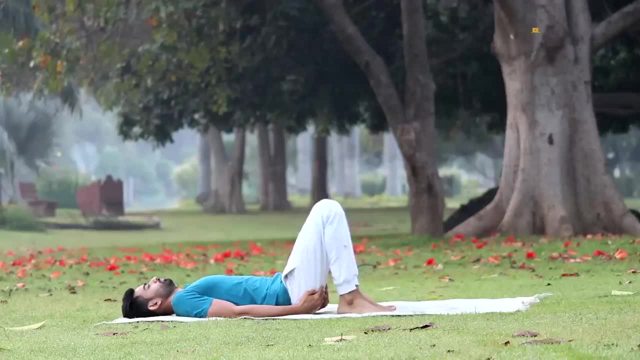 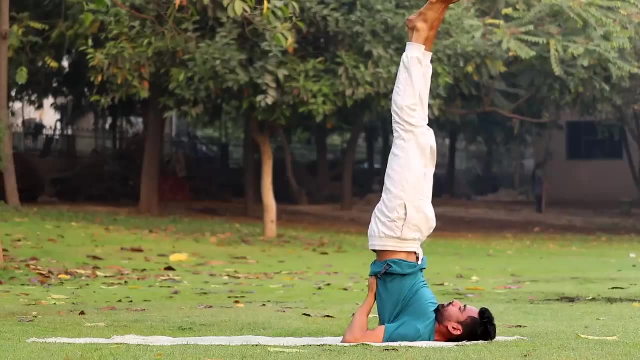 Ardha halasana with one movement. lift your legs, buttocks and back so that you come up high on your shoulders. support your back with the hands. your weight should be supported on your shoulders and upper arms in the same way. you can do the same with the other side of the body, so that your 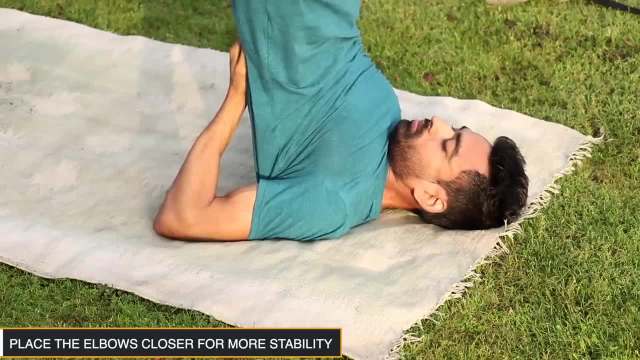 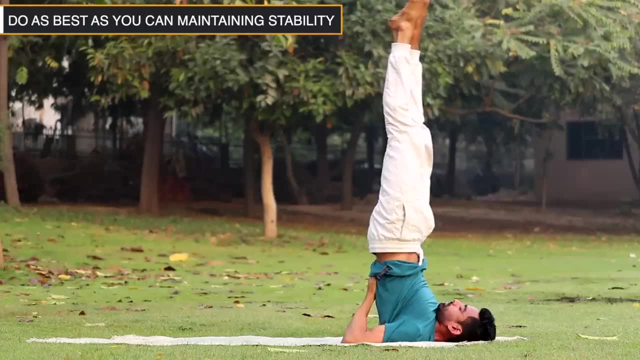 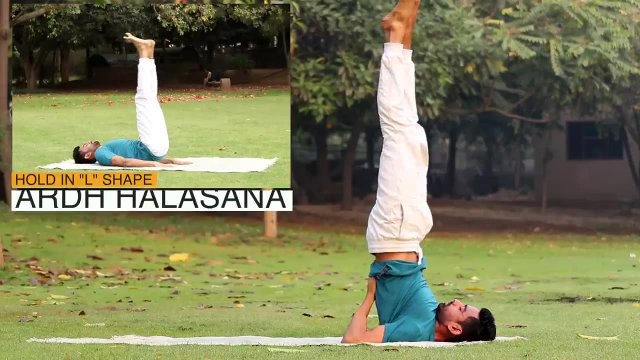 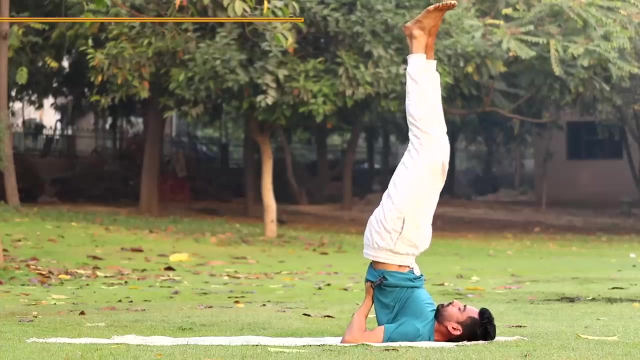 shoulders and not on your head and neck. lift your heels higher, as though you are putting a footprint on the ceiling. keep breathing deeply as you hold this pose for about 15 seconds for Ardha halasana. hold your body like that in L shape: brain power, face glow, thyroid function. sarvangasana is highly effective now. 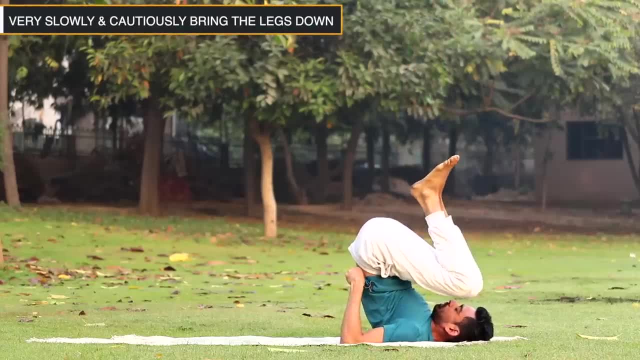 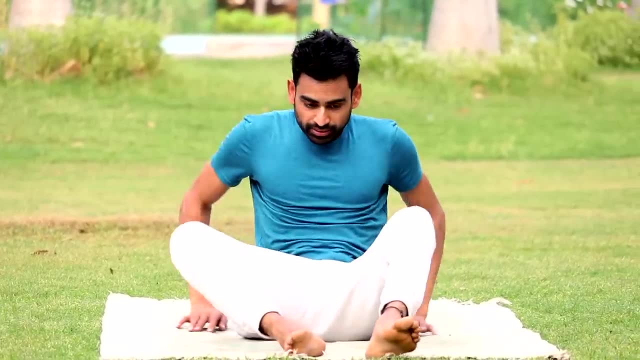 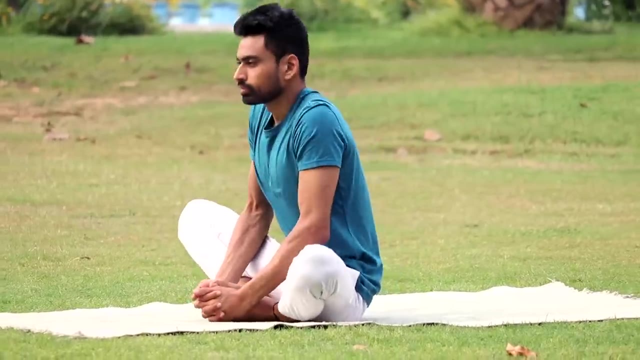 without lifting the head. slowly bring your spine down completely to the floor. relax for a few seconds. feel the sensations within your body. next is baddha konasana, popularly known as the butterfly pose. sit with your spine erect. now bend your knees and make an effort to bring the heels as close to the 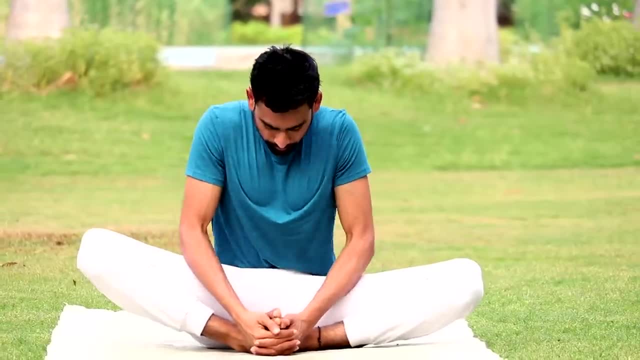 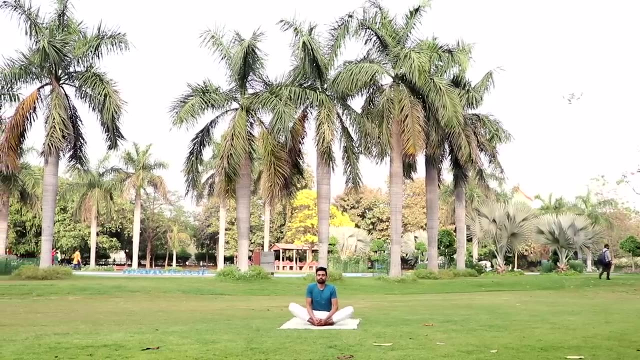 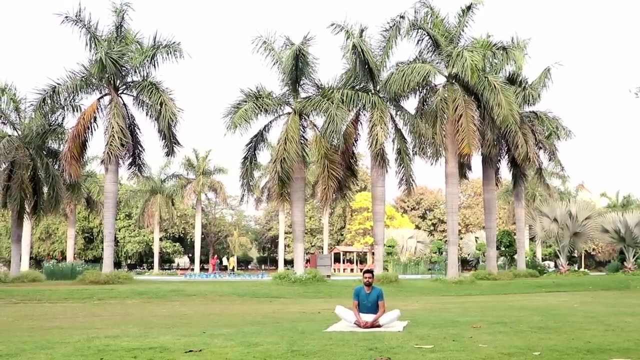 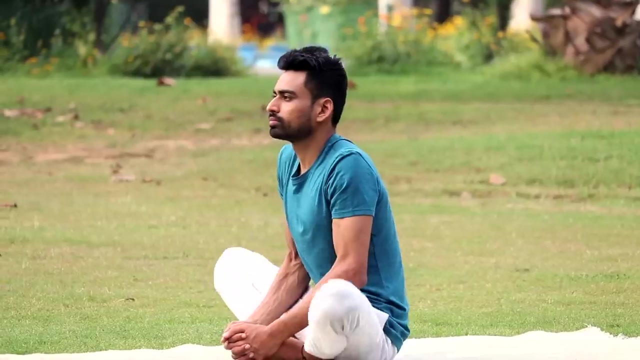 genitals as possible. do it comfortably, as much as your body allows. now take a deep breath in, breathing out. start flapping both the legs up and down like the wings of a butterfly. flap comfortably at your own pace for about 30 seconds. keep breathing normally throughout. you can instantly feel the stretch. one of the best asanas for. 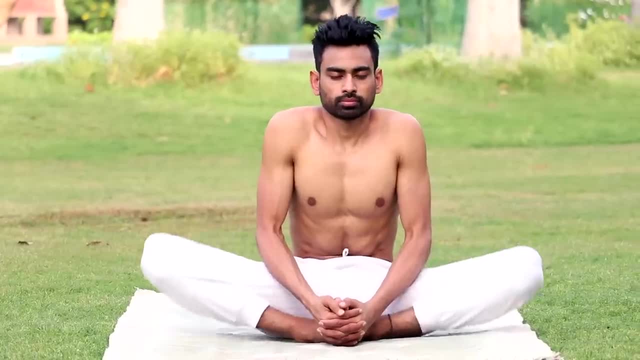 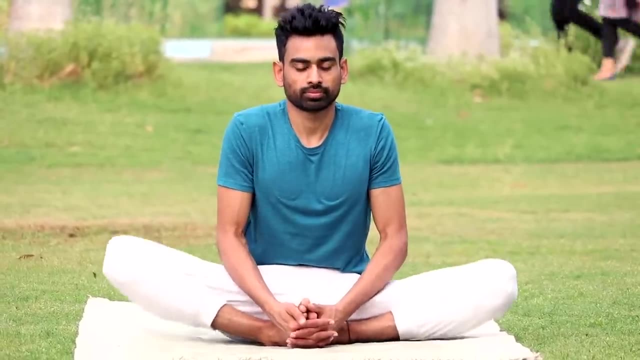 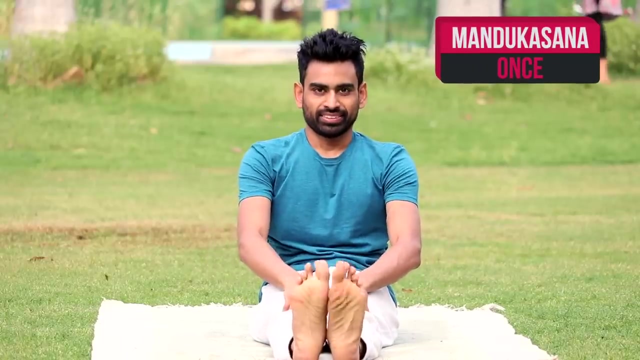 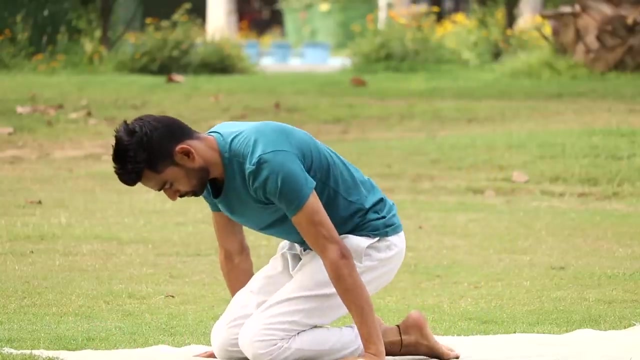 strengthening the pelvic region. it is highly recommended in PCOD and the problems related to menstruation and prostate. relax by straightening the legs out in front. moving on to the last asana, the mandukasana or the frog pose the ultimate asana for diabetes. first of all, sit in vajrasana. 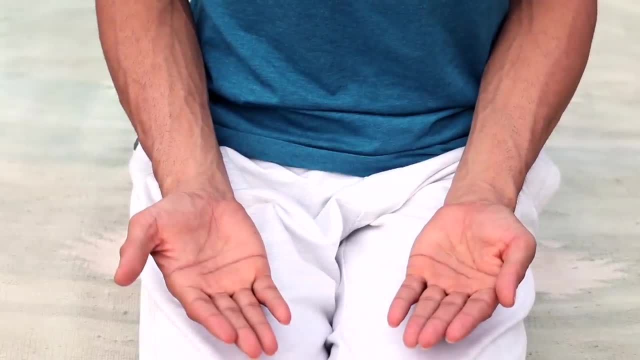 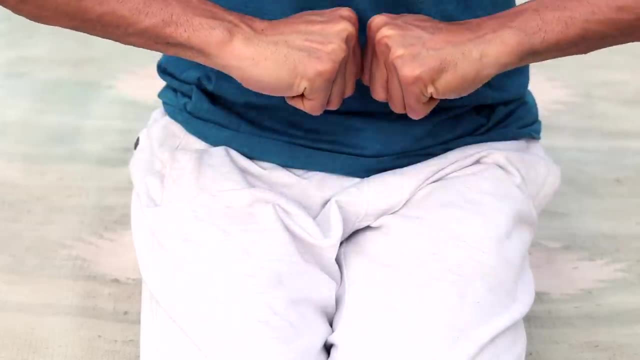 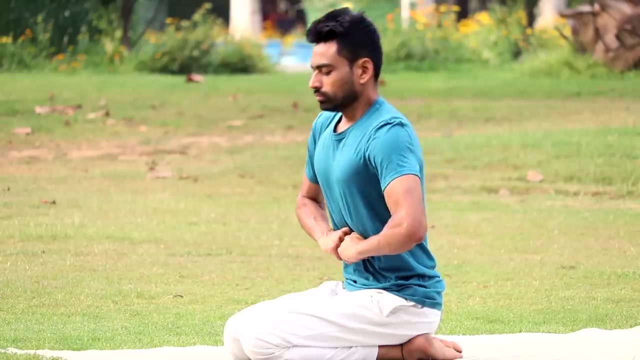 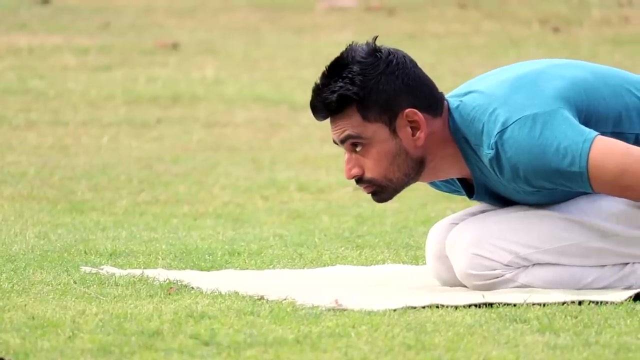 place your palms on the thighs facing the ceiling, keep the thumbs inside and make fists with both hands, like that now. place your fists firmly on the adjacent side of belly button, just like that now. take a deep breath in, then exhaling it out. bend downward, hold your position close to the ground, look in front, hold your breath in this. 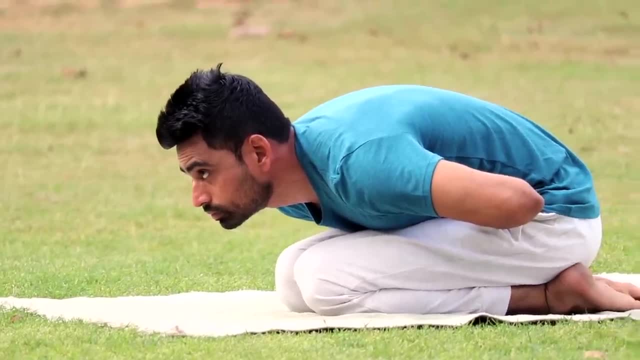 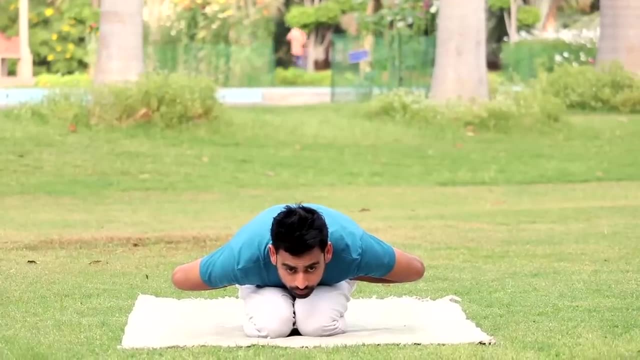 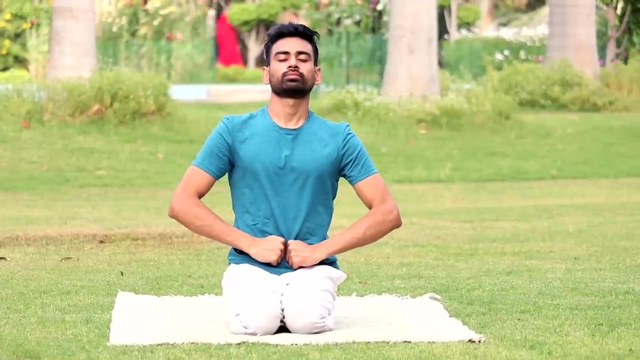 yoga posture for a few seconds, comfortably, without straining, feel the pressure exerted. mandukasana exercises many important organs like pancreas, gallbladder, liver and spleen, then slowly come up with inhalation, back to the original position, relax. so these were the six yogic postures, especially. designed for our business. students who want to give a shout out to our monthly asana sports training videos, stay tuned to our website and follow the links in description to make sure you stay up to date with the videos on all the videos of this video and what you are doing with your classes activities. hope to see you in the coming weeks. bye, bye, y'all. 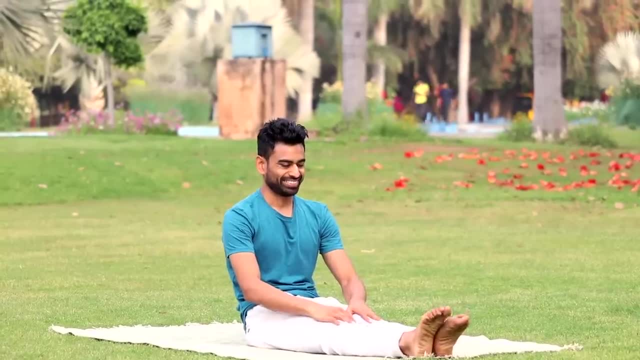 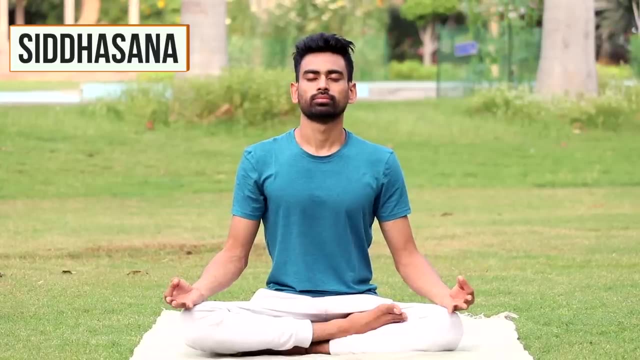 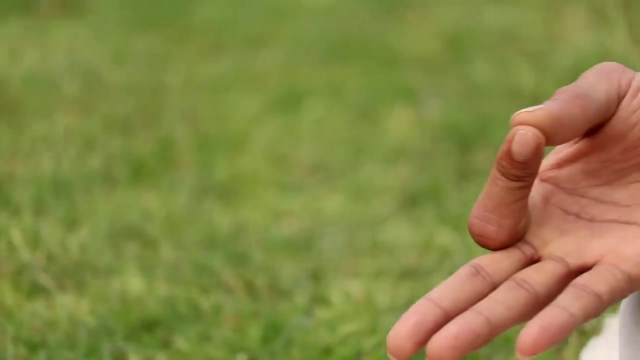 modern lifestyle Well done. Now let us do breathing exercises. Sit straight, either in Sukhasana, Ardha, Siddhasana, Siddhasana or Padmasana, Whatever you are comfortable in. Spine should be erect. neck straight, hands in Dhyan Mudra. Smile on. 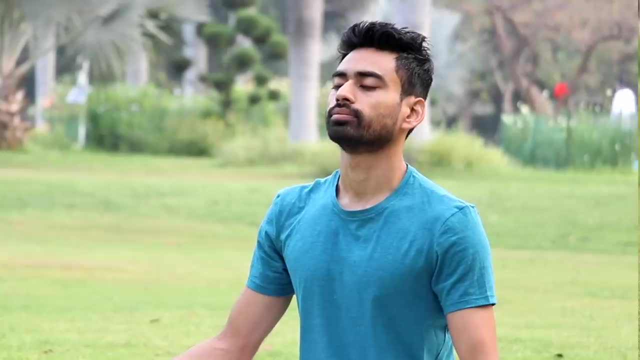 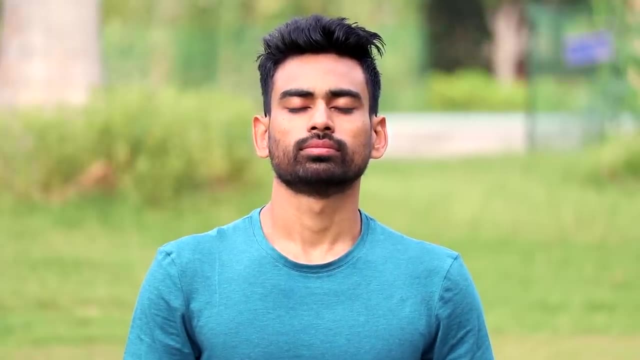 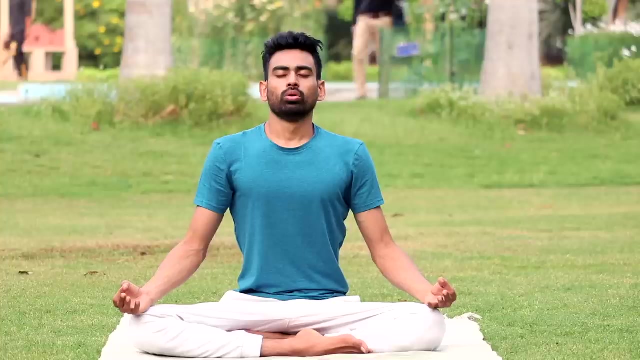 the face radiating positivity. We will begin with chanting Aum three times. Close your eyes with a mild focus in between your eyebrows, Take a deep breath in and slowly chant Aum. Aum is not a sound related to one particular religion. It is the primordial. 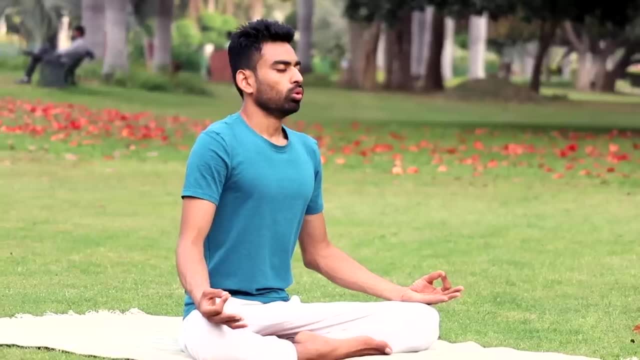 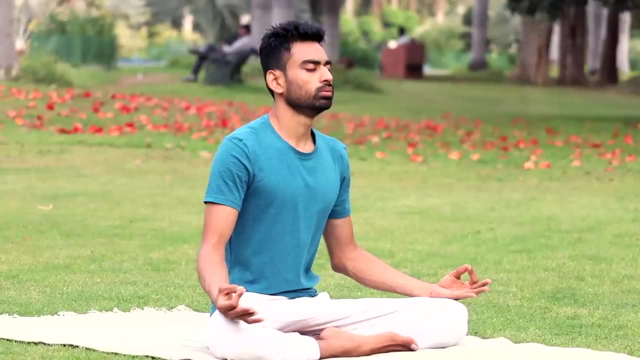 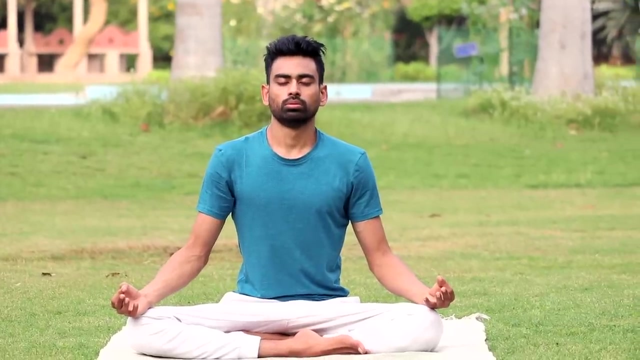 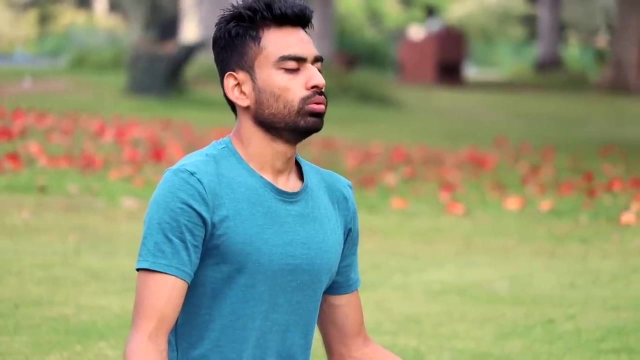 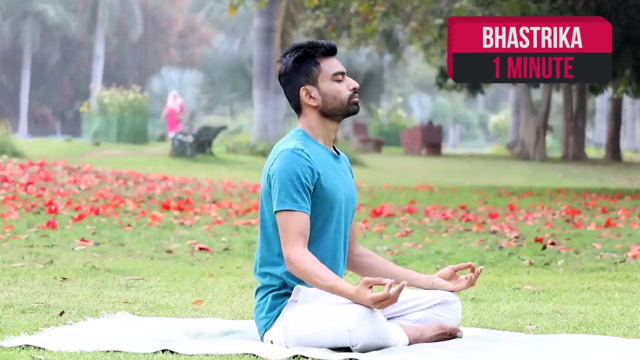 sound of the universe. Aum refers to Atman, our self within and the Brahman, the ultimate being Aum unifies Atman with Brahman. The vibrations of this divine sound balances the body within. cleansing the aura. Now we will do. Bhastrika or Bellows, breath Back straight, eyes closed, Take a deep breath. 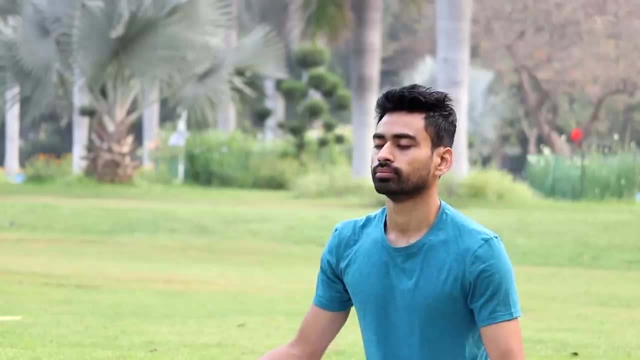 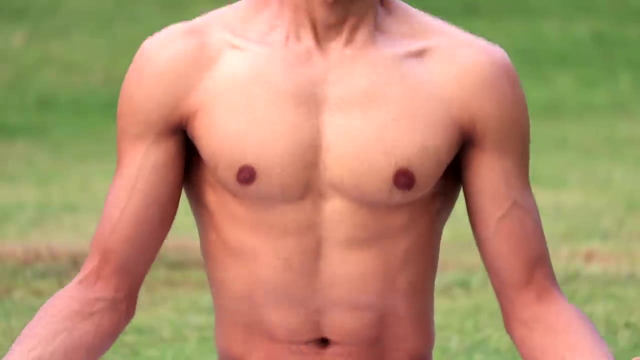 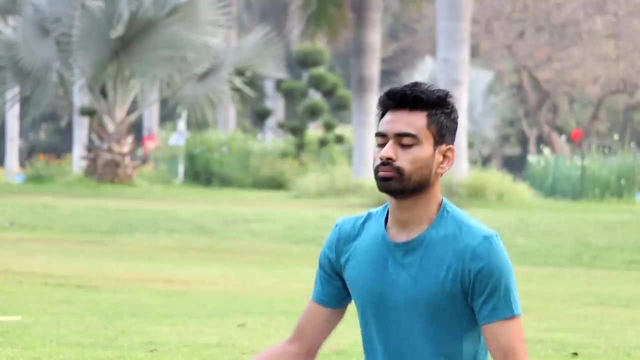 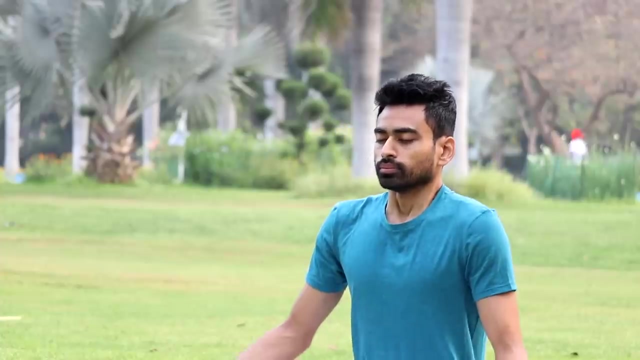 in through your nose and then exhale slightly forcefully through your nose. We will do this for a minute With smile on face. with each deep inhalation, feel that the pranic energy from the universe is entering your body And with each exhalation, feel that the negativity impurities are flowing. 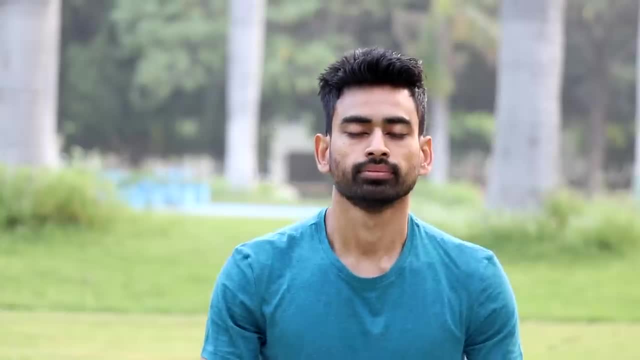 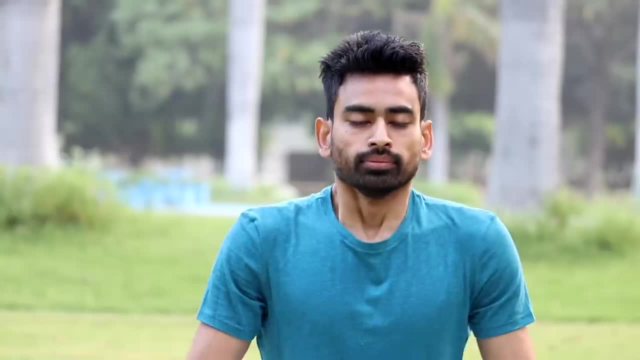 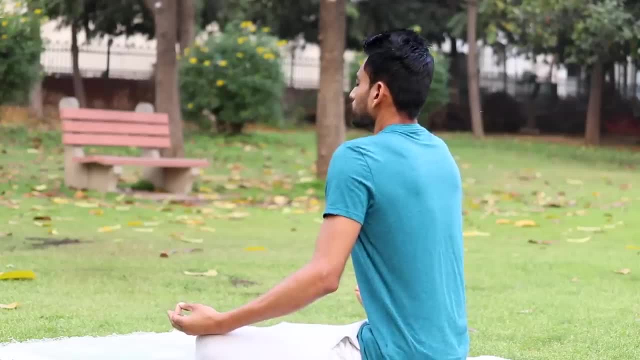 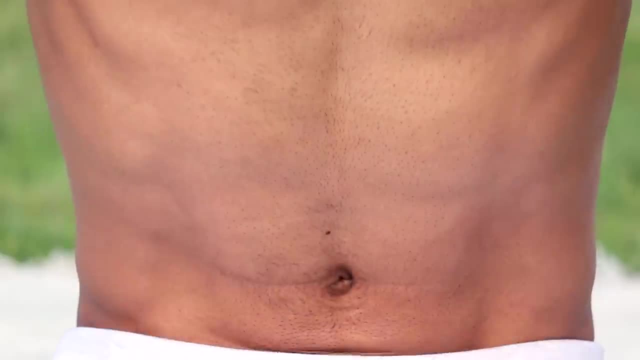 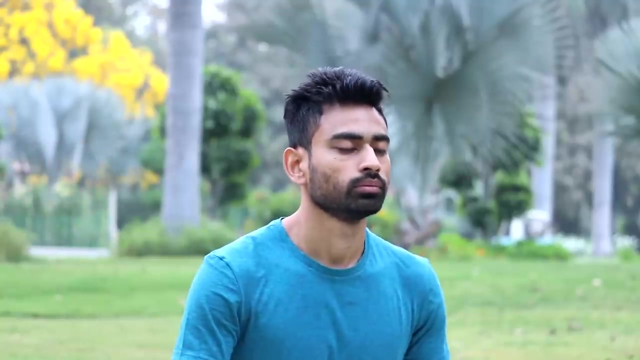 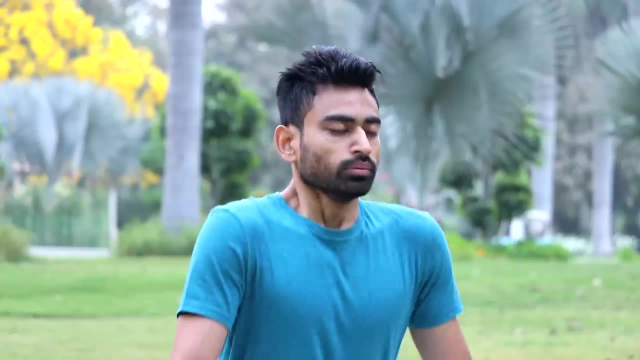 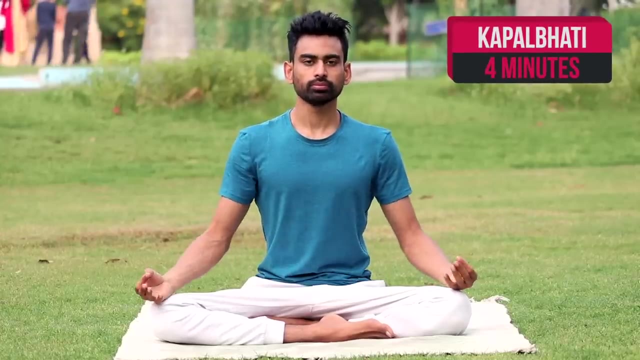 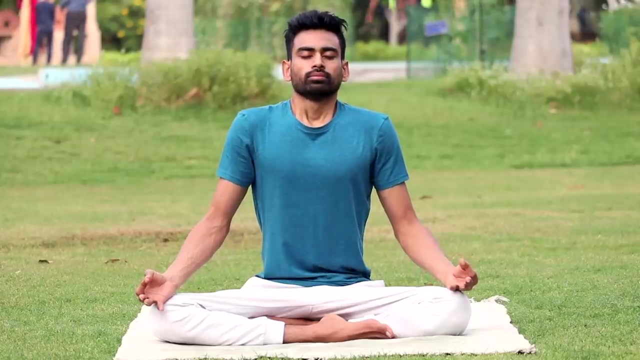 person that block his or her evolution. Now we will do Kapalbhati, or rapid exhalation, for 4 minutes. Back straight, eyes closed, body relaxed, mind calm. Take a deep breath in and then expel the breath with forceful contraction of the abdominal. 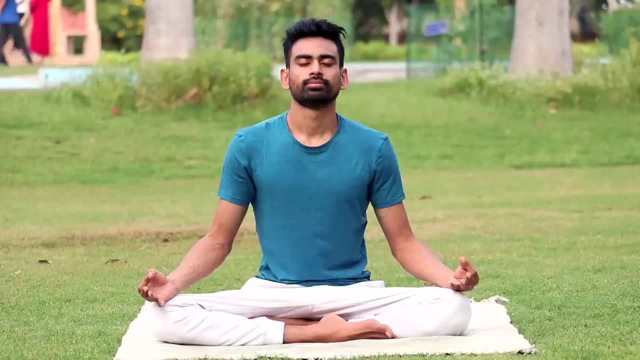 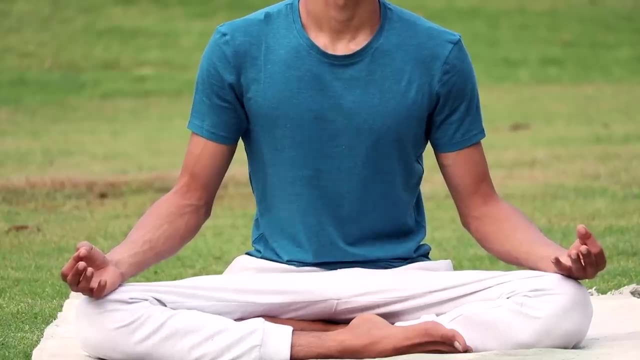 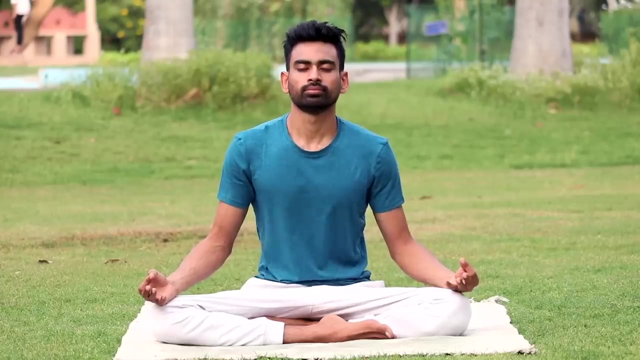 muscles. Yes, just like that. Throughout this Kriya, try to keep a mild focus on your stomach area. Do not worry about inhaling, just focus on exhaling. The point between two exhalations is when your body will automatically breathe in. 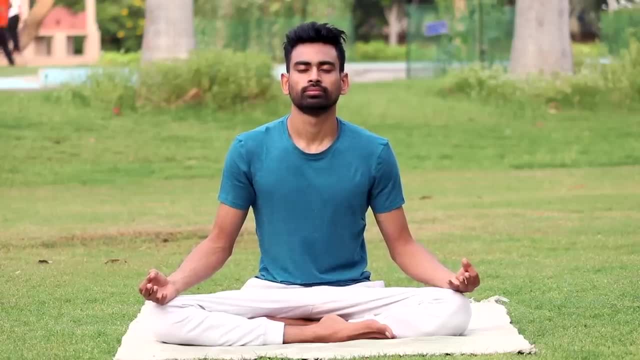 Its mechanism is similar to hand pumping the air in a bicycle. Here we are pumping breath out of the body. Kapalbhati literally translates to the shining forehead, And this is precisely what happens with regular practice of this yogi Kriya. 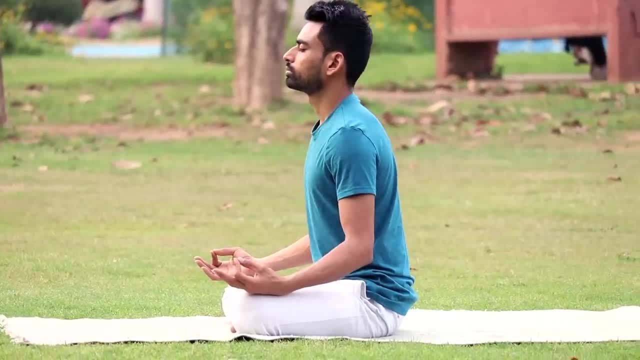 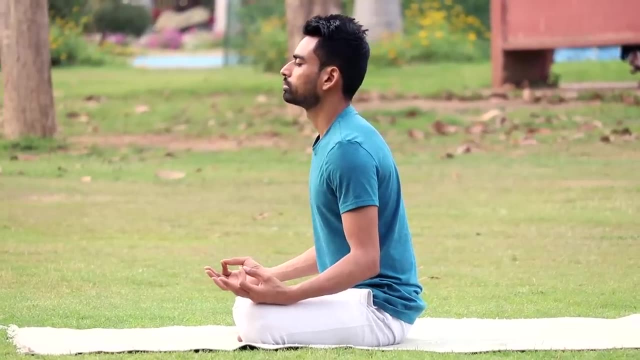 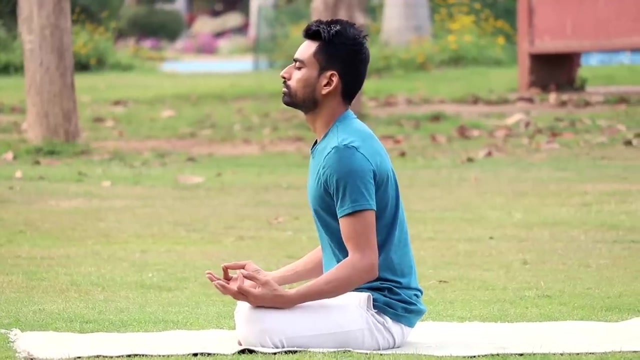 A forehead that glows not just from the outside but also from the inside, making the mind illuminated. Now we will do Kapalbhati, or rapid exhalation, for 4 minutes. Aim for at least 60 outward strokes of breath in a minute. 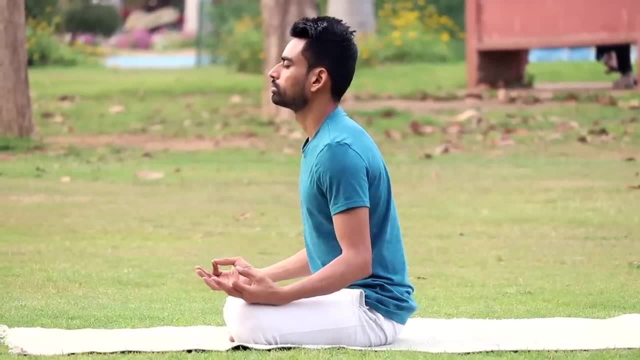 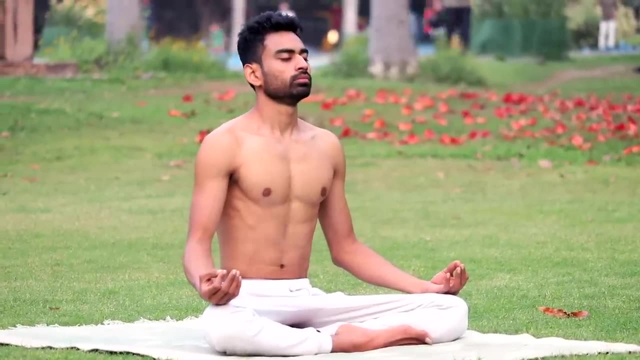 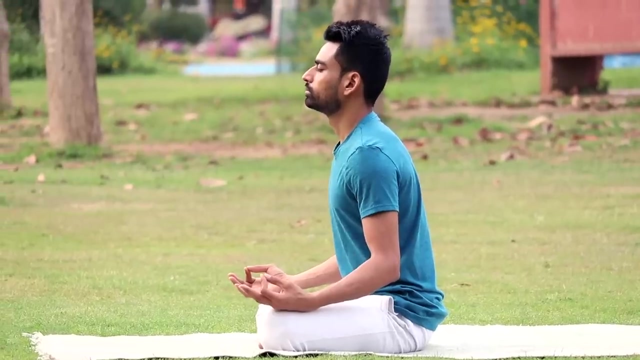 Slowly. you can increase this number to 70,, 80 or even in 3 digits. Progress slowly, There is no hurry. You can even count the exhalations in mind, if you so wish. With every outward breath, Feel that you are pushing the toxins out of your body. 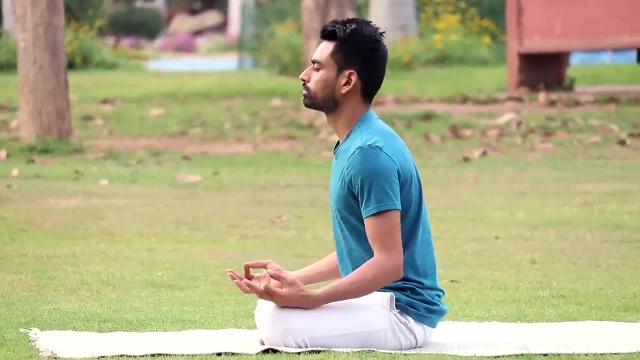 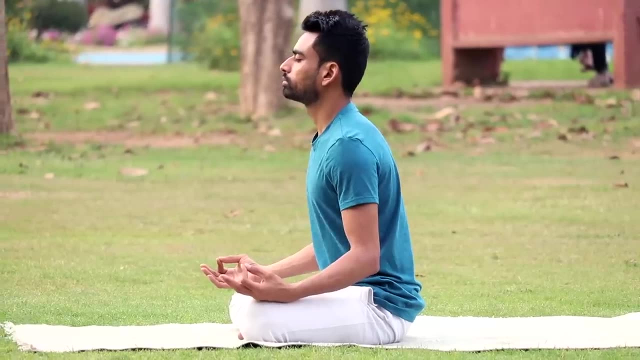 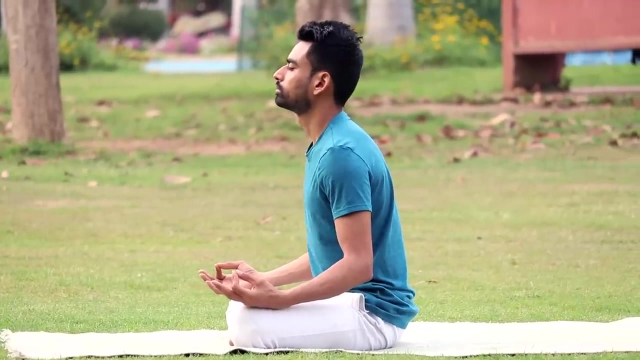 Your digestive system is being exercised, Your heart is pumping better, The liver is functioning better, The internal factory is being getting cleaned up, The workers are at work and you are simply facilitating them. The regular practice of Kapalbhati Pranayama detoxifies all the systems in our body. 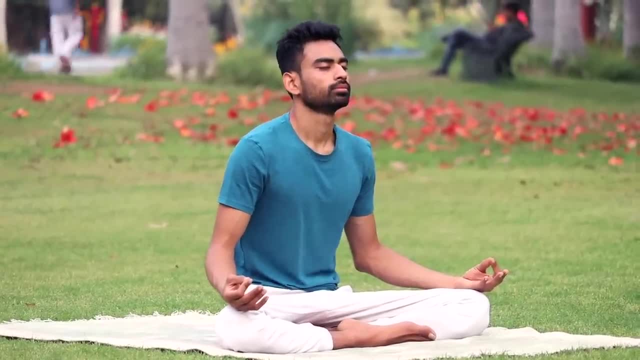 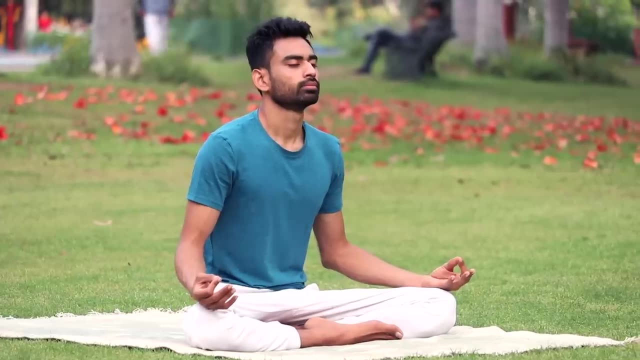 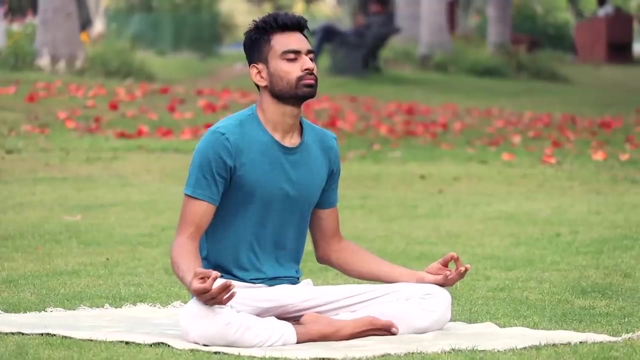 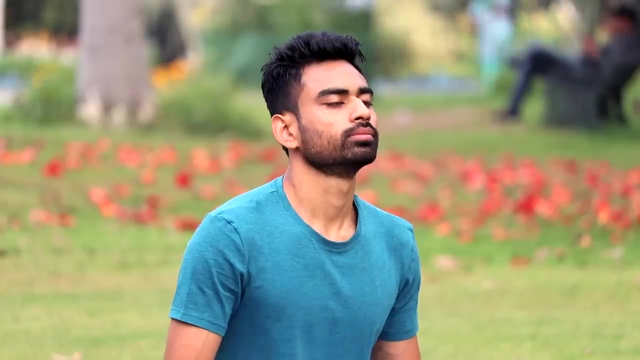 This is a very important practice. It is a very important practice. It is a very important practice. It is that powerful Fat loss is just a byproduct. Just like milk gets boiled faster if it is provided constant heat, The benefits of Kapalbhati are enhanced if it is done without a break. 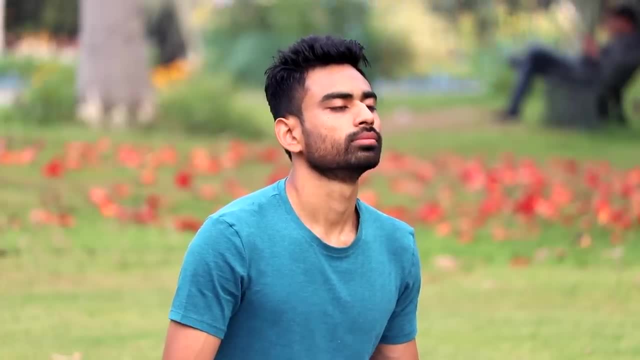 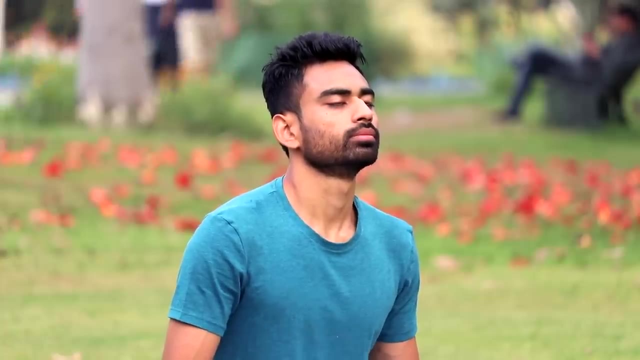 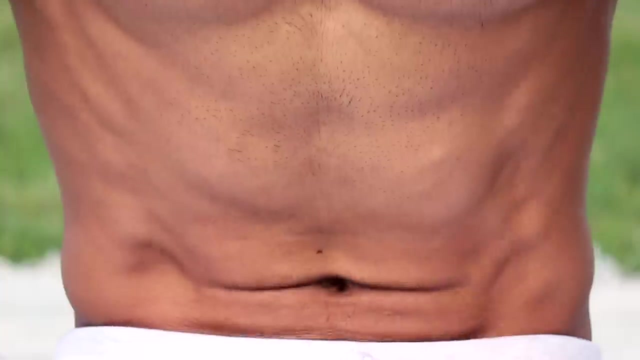 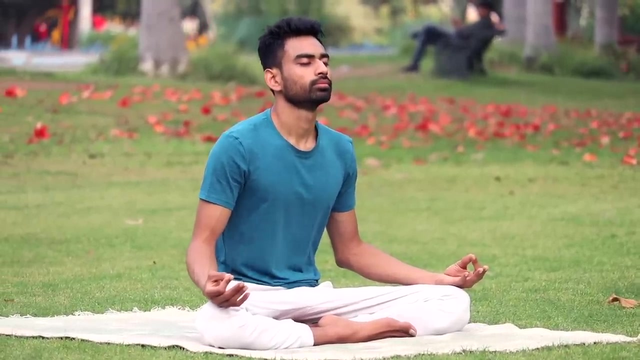 However, at no point over exert yourself. If need be, take rest for a second And then stop And then start again. In terms of circulating the blood, it is so effective that often it's compared to running. Kapalbhati has an energizing effect on the nerves and a refreshing effect on the brain. 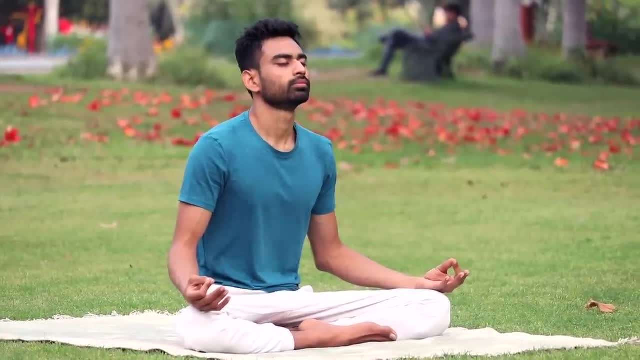 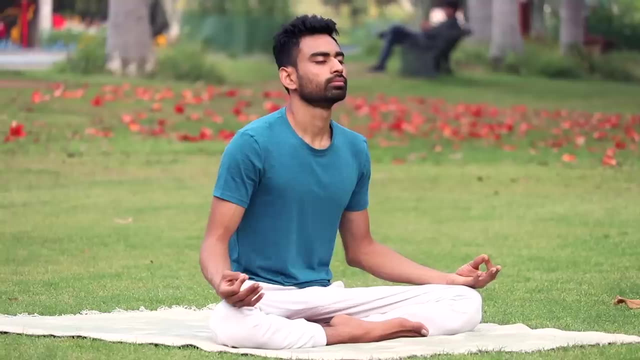 It strengthens the digestive system like no other Gas. acidity, indigestion, low appetite, malabsorption, you name it. Daily Kapalbhati practice alone has a powerful effect. It strengthens the digestive system like no other Gas. acidity, indigestion, low appetite, malabsorption, you name it. 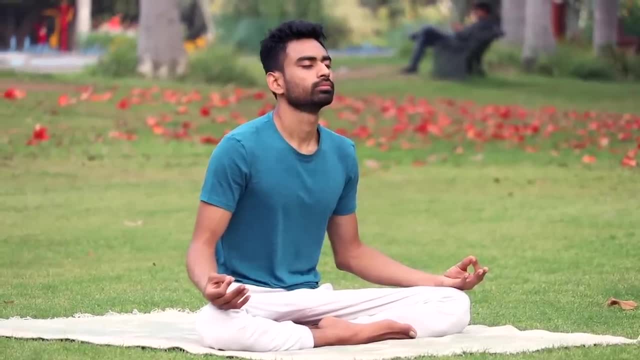 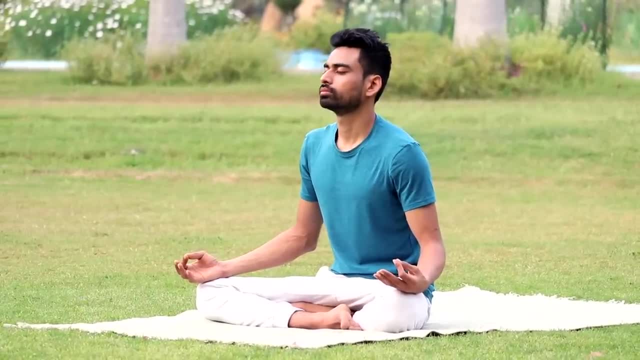 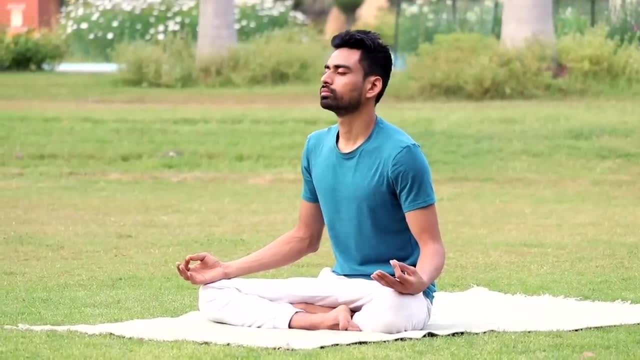 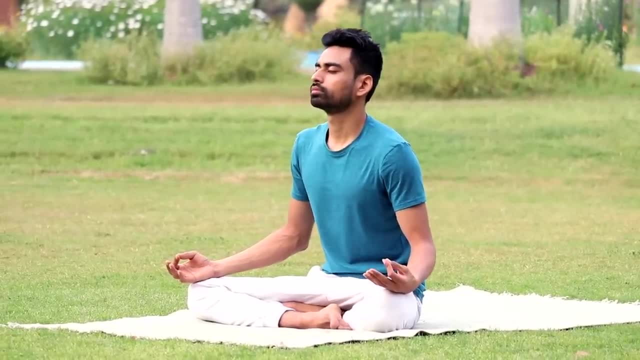 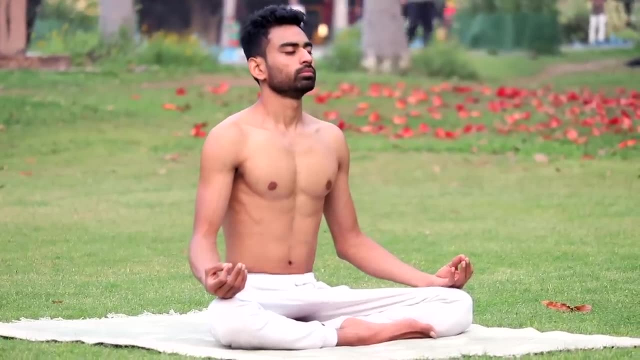 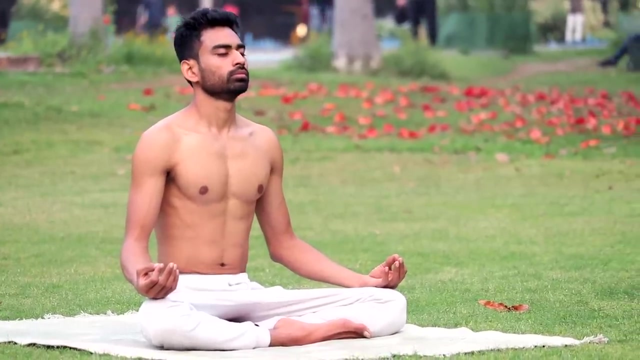 It's the middle portion that remains largely unmoved. That's where most diseases arise from Kapalbhati. doesn't let that happen. Kapalbhati naturally purifies the blood as well. That is why it is said that it keeps the face young and radiant. 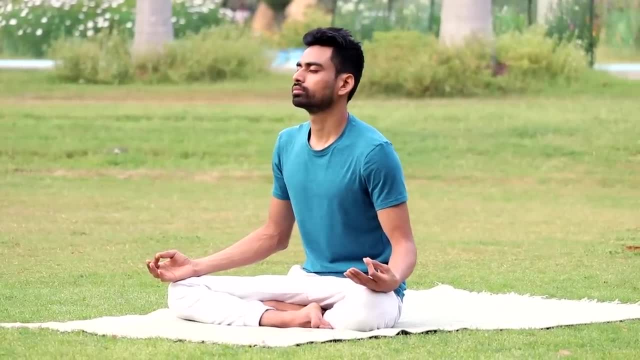 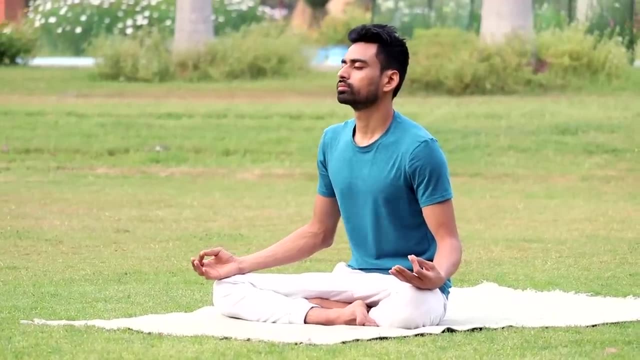 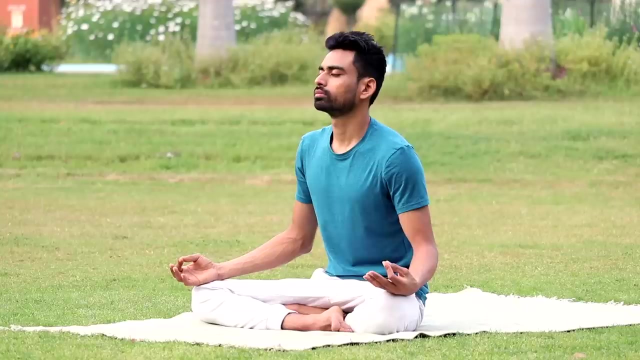 The 72,000 nadis, or subtle channels that make our human body. the Kapalbhati has the capacity to stimulate and clear their passage. Yogic pranayama is all about doing it with a calm, cheerful mind, with utmost faith and involvement. 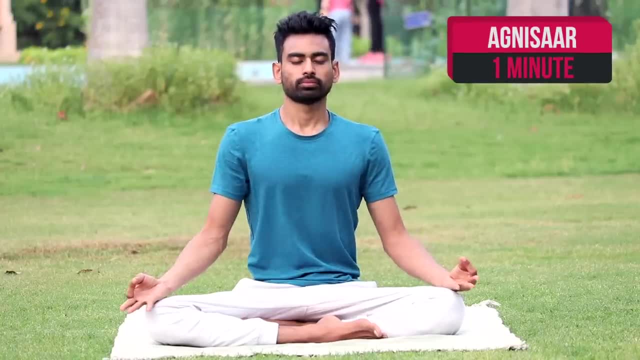 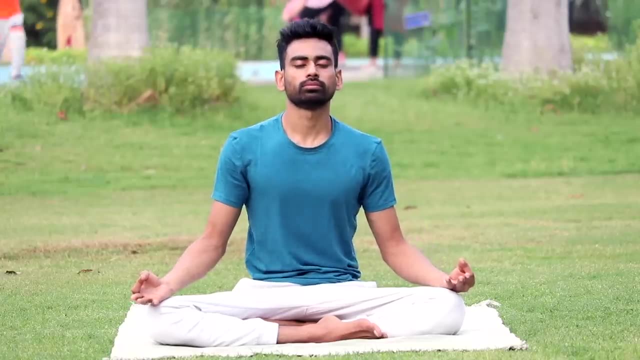 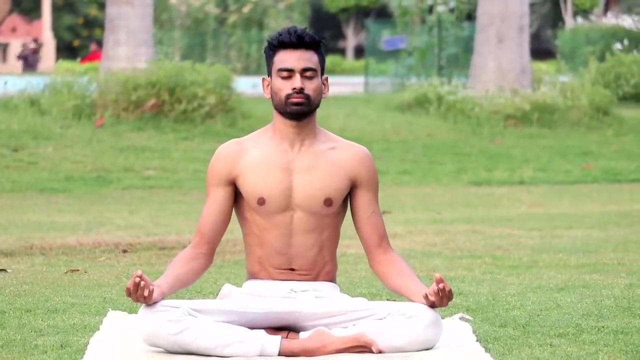 Now let us do Agnisar. Take a deep breath in, then exhale completely. Now contract and expand the stomach as many times as you can. 10 times is a good number for a start. Slowly you can increase this number to even three digits. 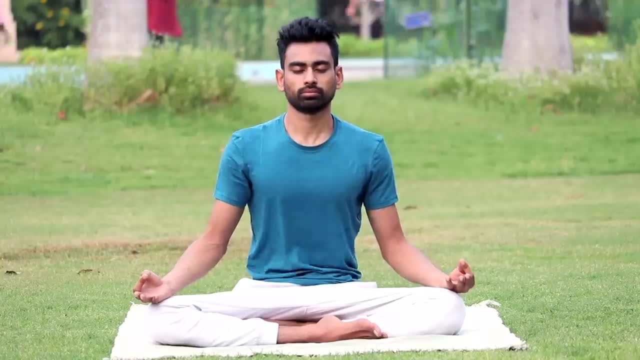 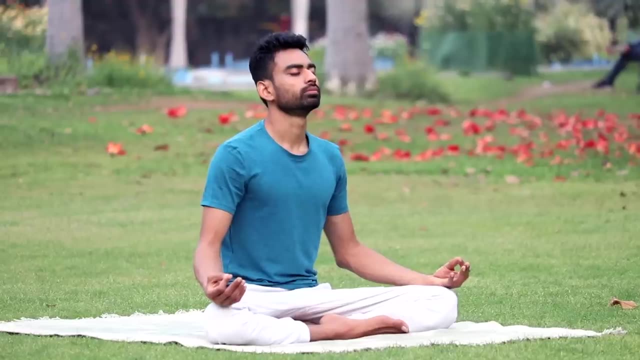 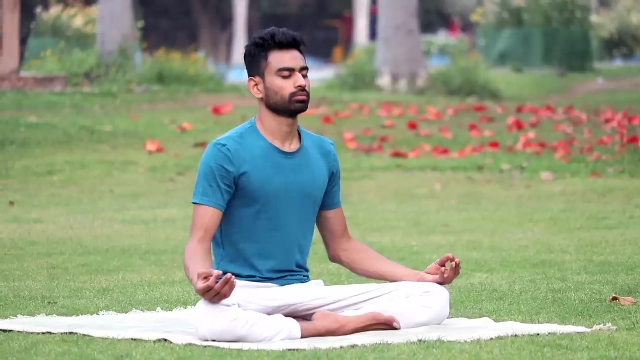 The positive impact of Agnisar is multiplied when done after Kapalbhati. Do it for one minute. The name Agnisar is derived from two Sanskrit words: Agni, meaning fire, and sar, meaning to flush. Agnisar kriya mainly affects the belly region and 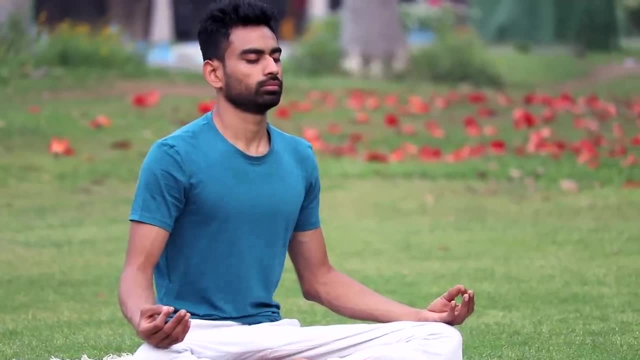 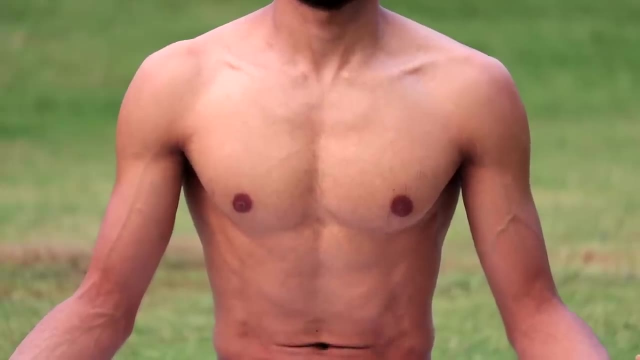 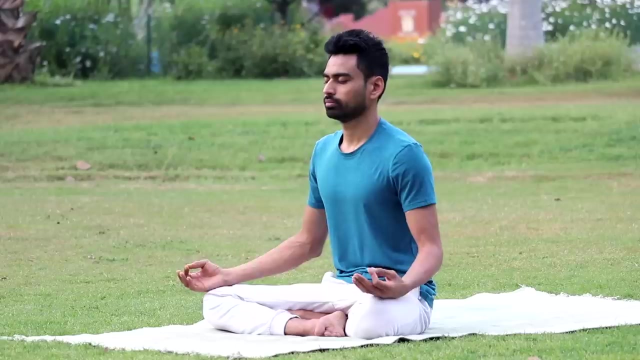 regulates the fire element in the body around the stomach and thus improves the process of digestion and relieves problems related to the stomach. It is said to balance the Manipur chakra near your belly. Next we will do Jalandhar Bandh, also called the chin lock. 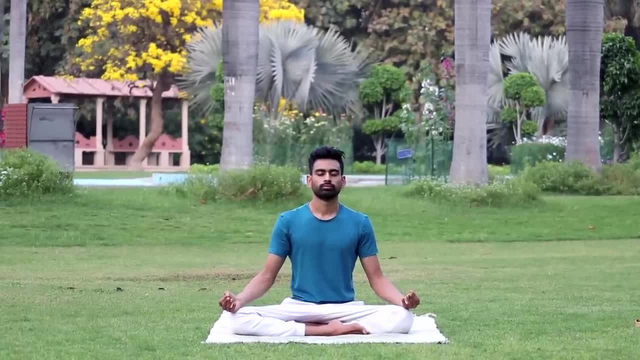 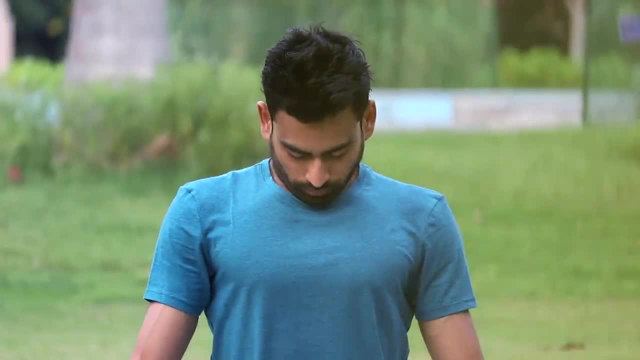 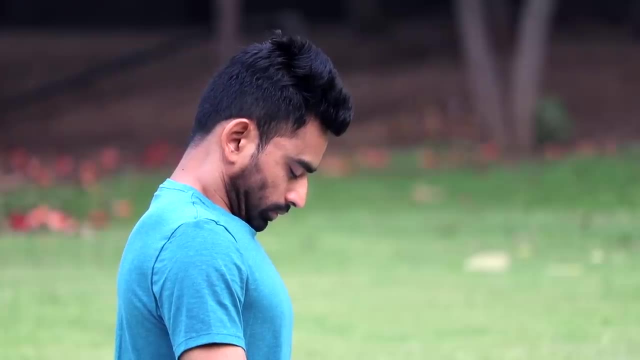 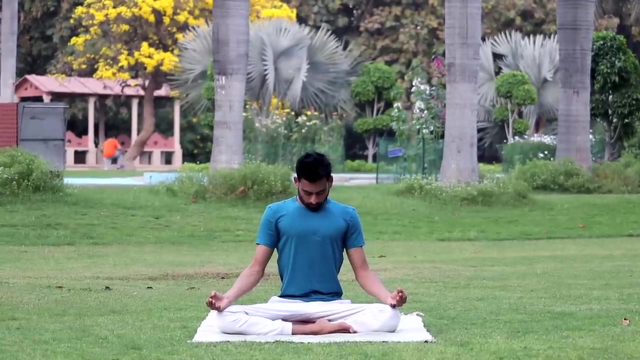 Inhale slowly and deeply through the nose. Now hold the breath, contract the throat and gently press the chin downward, almost touching the upper chest. Hold the bandh for as long as it is comfortable, Then relax the throat, raise the chin and exhale slowly through the nose. 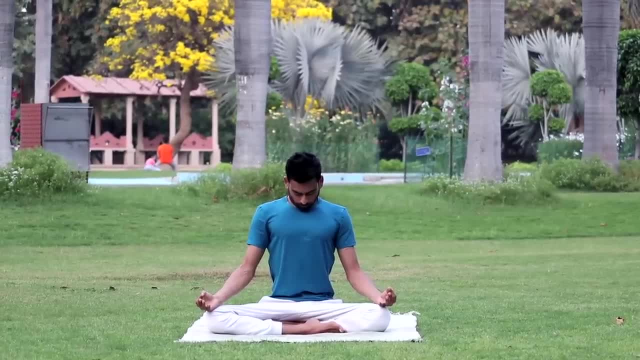 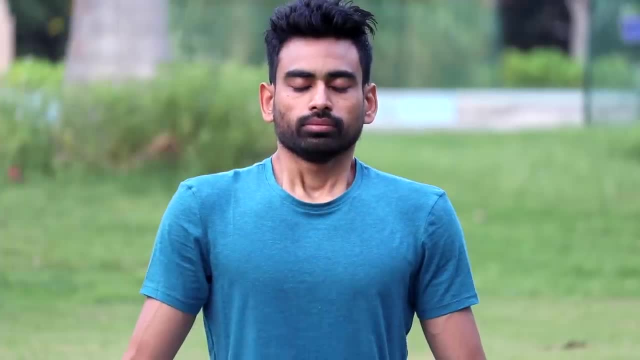 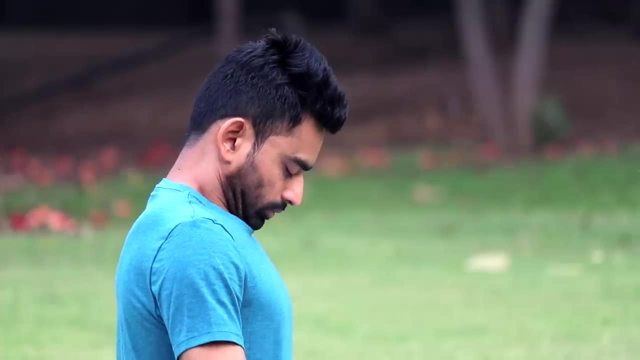 Do it three times. In yogic lore, Jalandhar Bandh, is considered of prime importance In getting over addictions of the body as well as the mind: alcohol, smoking, excessive masturbation, even addiction to sugar and junk foods. Whatever may be your concern, take it as a thought and do this bandh. 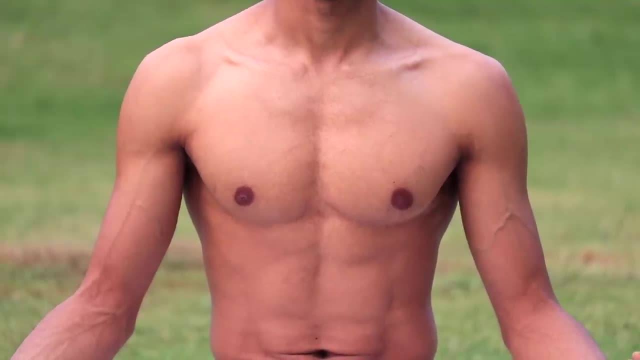 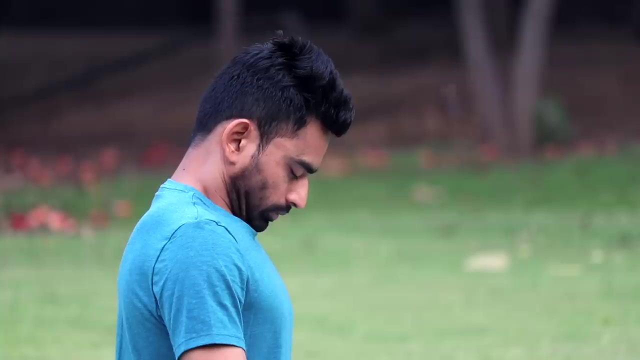 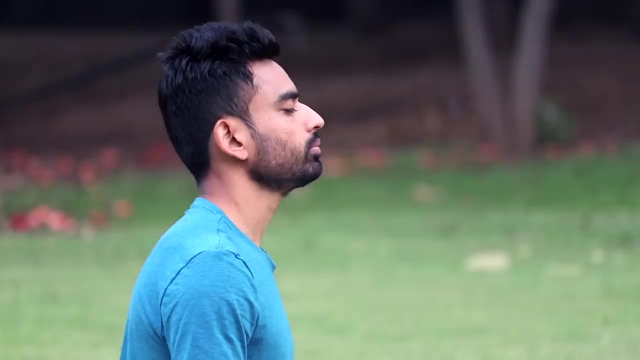 It tremendously increases the willpower With regular practice of Jalandhar Bandh holding breath for long times. it even stimulates the vagus nerve Mentioned in Maharishi Patanjali's Ashtang Yoga. its practice gives an instant gratification. 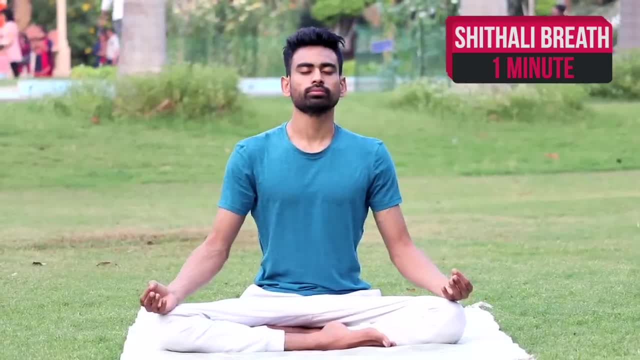 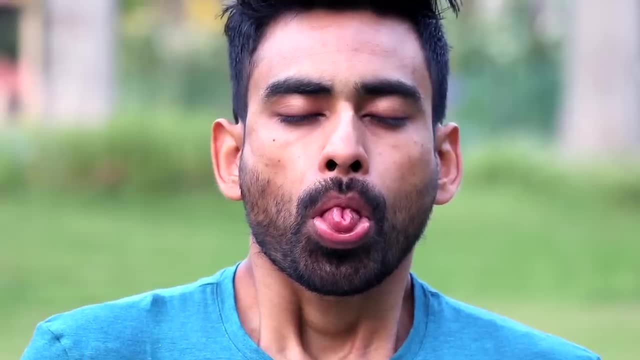 Next we will do the Sheetali breath. Keep the spine upright, eyes closed. Now bring your tongue all the way out. Fold the sides of the tongue like a tube. Take a long, deep inhalation through this tube. After the inhalation is complete, close your mouth and exhale through the mouth. 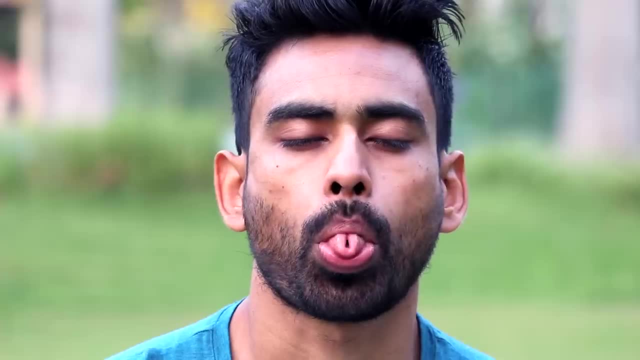 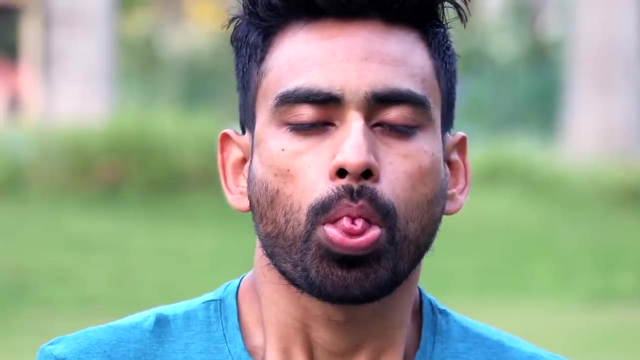 This is the best way to do it. It is a very effective way to get rid of constipation. This is the best way to get rid of constipation. As the name suggests, it cools down the body, soothing internal inflammations. 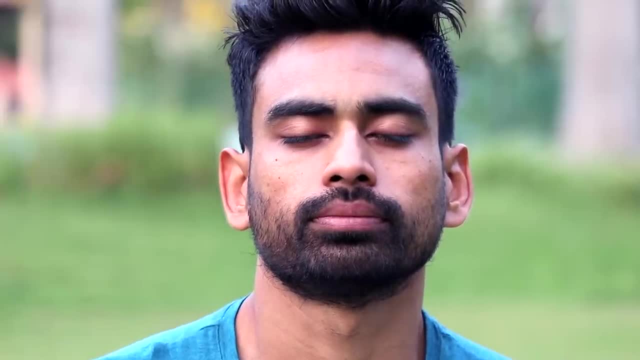 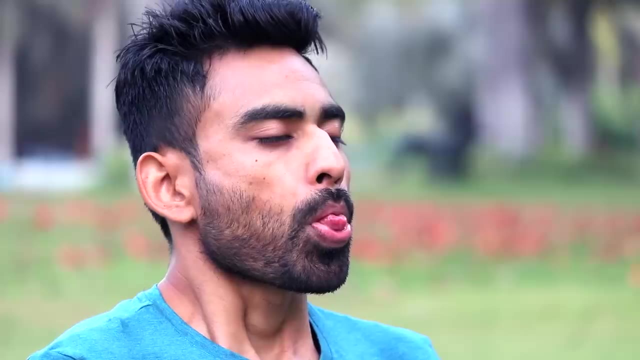 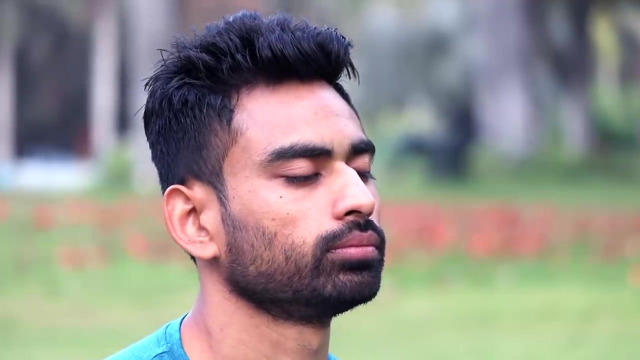 Can you feel the instant cooling effect? Let's do this for a minute. In the scorching heat of India's tropical climate, Sheetali breath is a useful tool to keep the internal body temperature in check. The cooling effect of Sheetali breath is penetrating and deep. 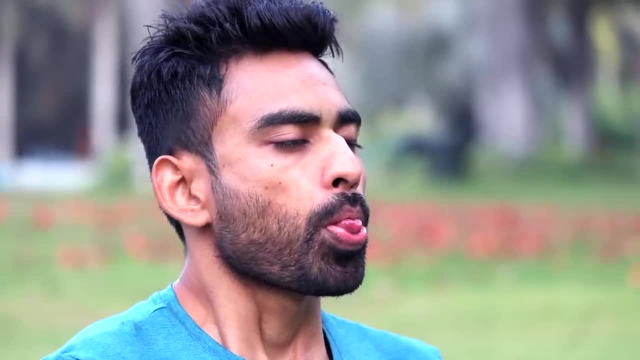 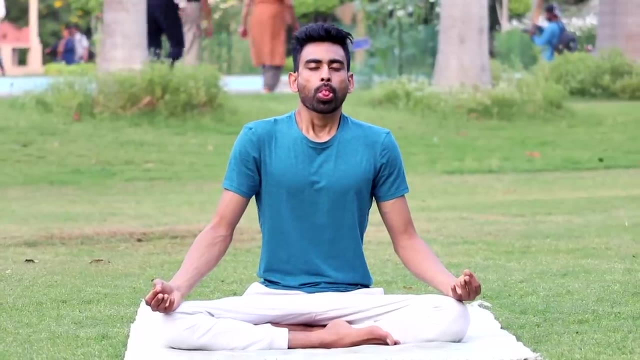 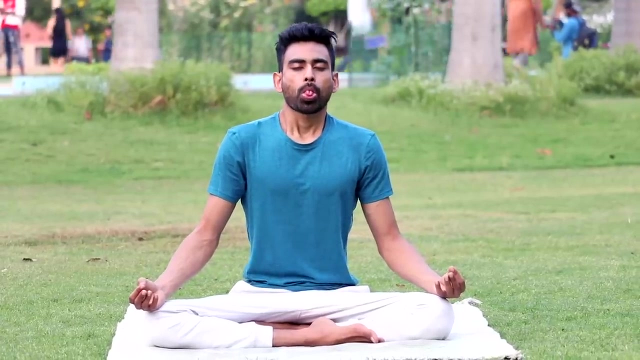 Any issues pertaining to the body: heat, ulcers, acidity, pimples, rashes, anger, stress. Sheetali breath has a healing effect. Feel the excess heat from your body getting flushed out. Cooling for the body. it rejuvenates the mind. 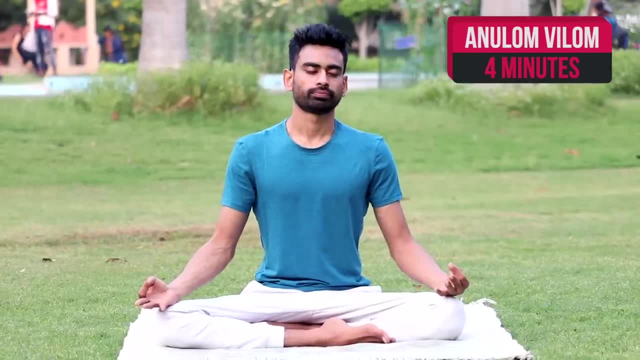 Now we will do Anulom Vilom, or alternate nostril breathing With your right thumb, close the right nostril. Now we will do Anulom Vilom, or alternate nostril breathing With your right thumb, close the right nostril. 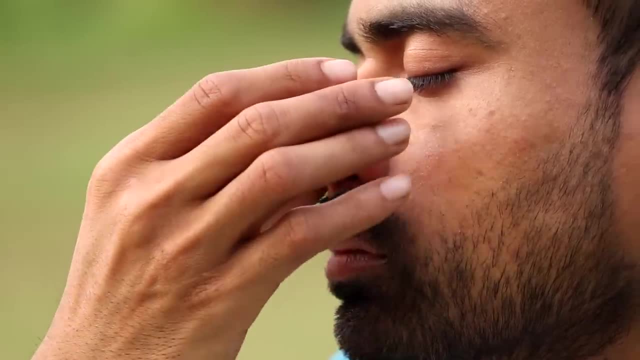 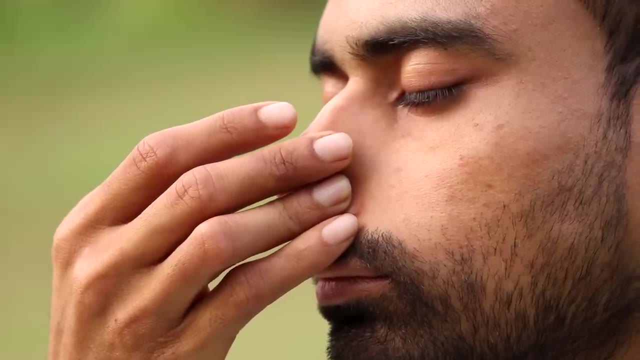 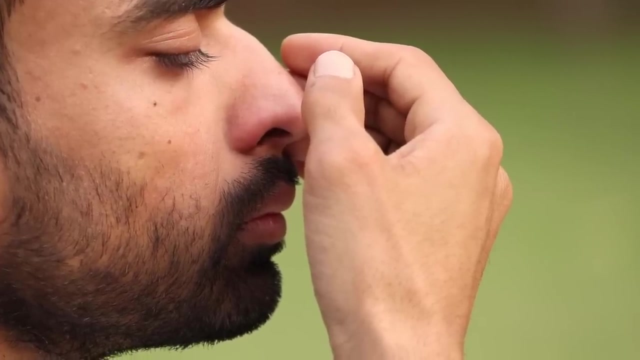 Take a slow, deep breath in through the left nostril, Place the middle two fingers closing the left nostril, and exhale slowly but completely through the right nostril In the same position. inhale deeply from the right nostril, release the fingers place. 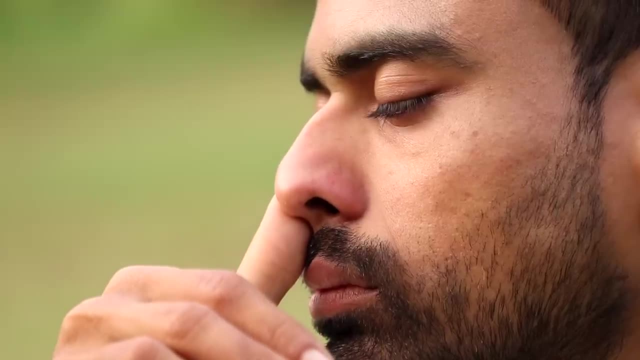 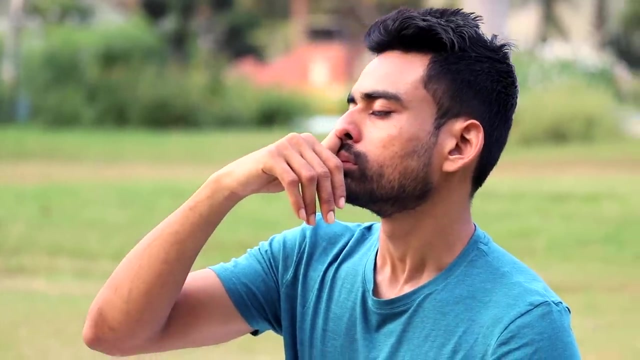 the right thumb again on the right nostril and exhale completely from the left nostril. This completes one circle of Anulom Vilom Pranayam. We will do this for a minute. We will do this important Kriya for 4 minutes. 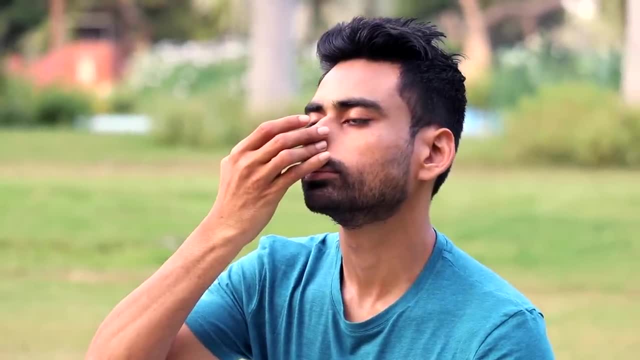 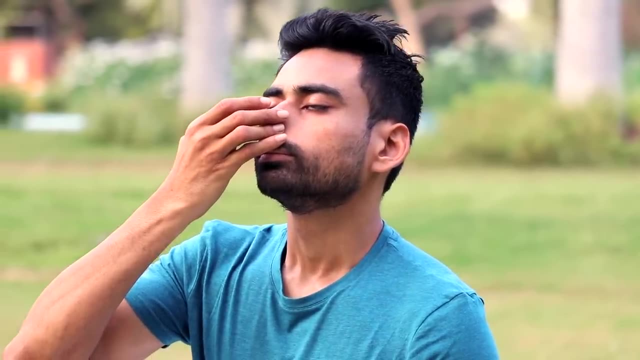 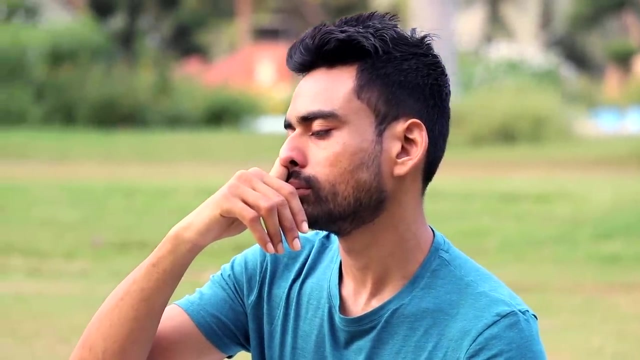 Do it slowly, keeping a mild focus in between your eyebrows. For deeper effect. take long, deep inhalations filling your lungs to their full capacity and then exhale slowly, completely. Try to keep the time of inhalation and exhalation roughly the same. 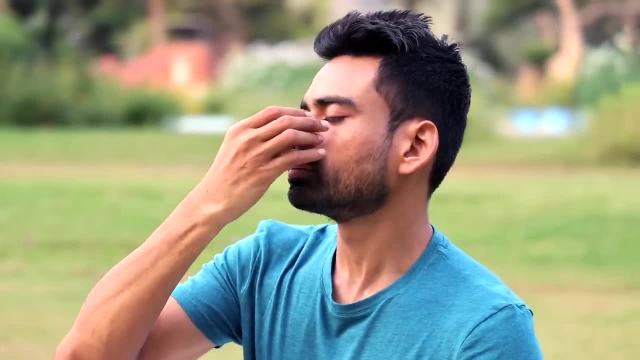 Anulom Vilom has earned the name of Anulom Vilom Pranayam. Anulom Vilom has earned the name of Anulom Vilom Pranayam. Anulom Vilom has earned the name of Anulom Vilom Pranayam. When di Crash Krathit has received chanaal, he returns to the Chandra. Chandra. It has a special universe, The different瞳 existing within a superlative. 모두 is an anna-a, anna-e and anna-a. 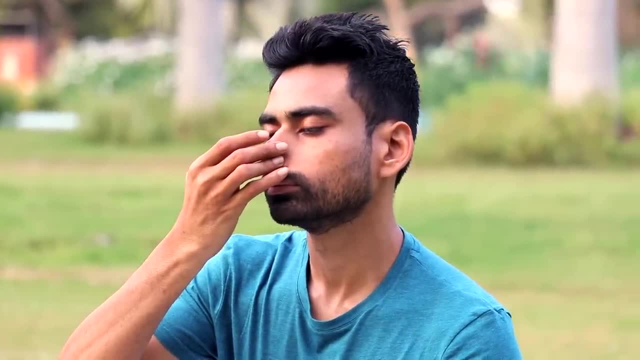 Concerning chrodsem pranayam naadi shodhan. pranayam Naadi, referring to chanal shodhan means cleaning and pranayam is the technique. Howama mental is called Praanayam. 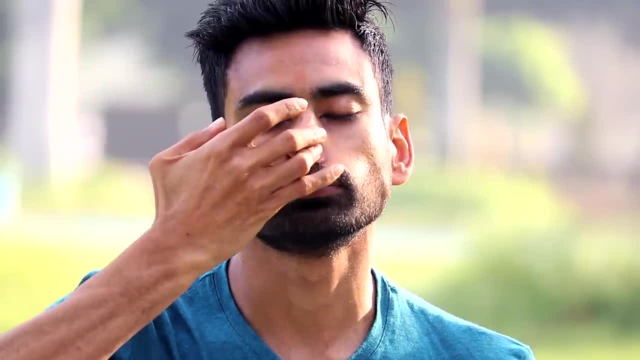 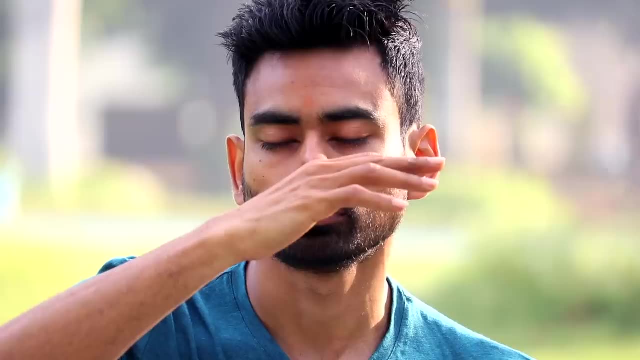 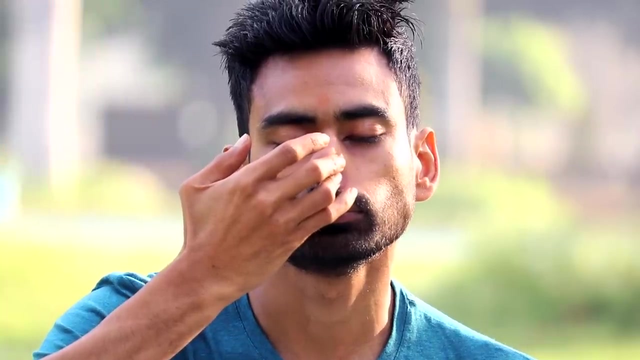 Ede, Pata and Pengla are two most important nadis in the human body. Ede, or the moon connector connecting the left nostril, corresponds to the right hemisphere of the brain. Pengla, or the solar chanal connecting the right nostril, corresponds to the left side. 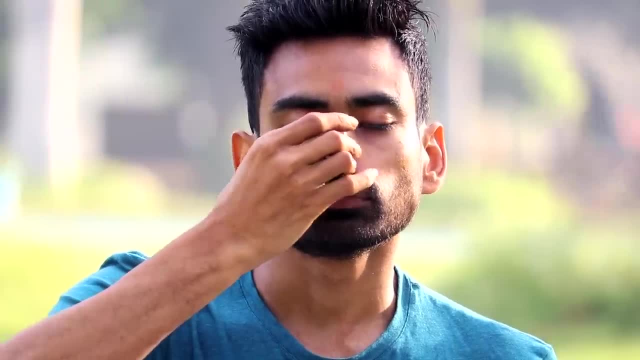 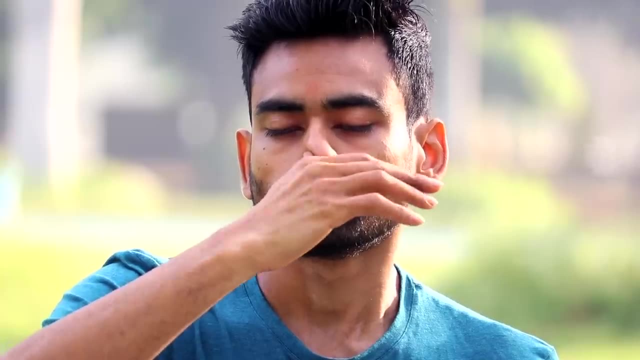 of the brain. Howama mental is also called Pranayam. When Anulom Vilom is practiced, these two nadis are cleansed. This brings about an equilibrium between the left and the right brain, which results in heightened states of awareness and perception. 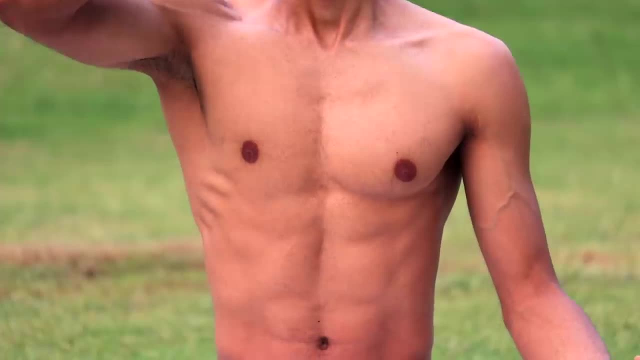 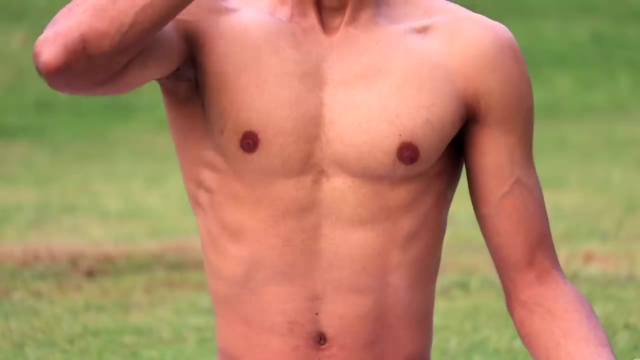 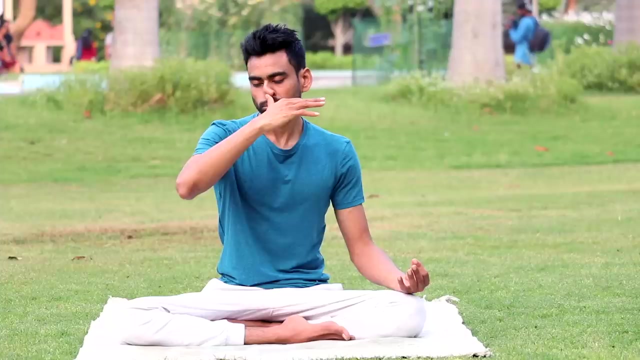 Physical health is then a byproduct. With every inhalation, feel the flow of prana entering your body, And with every exhalation, feel the impurities flowing out. Cleaning is going on at the deepest levels. It's no small feat. 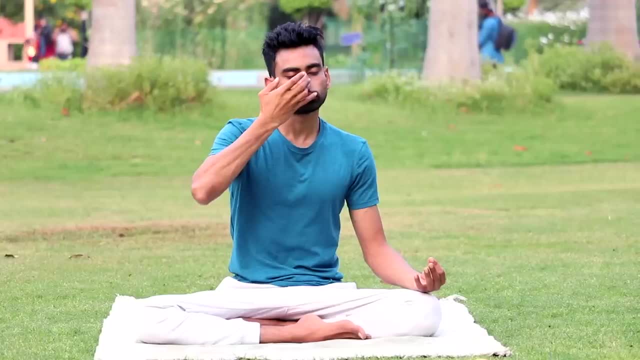 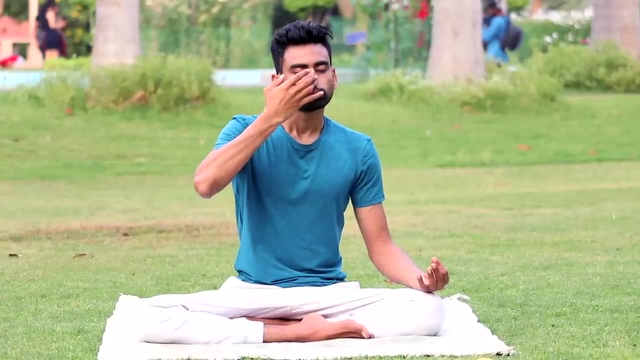 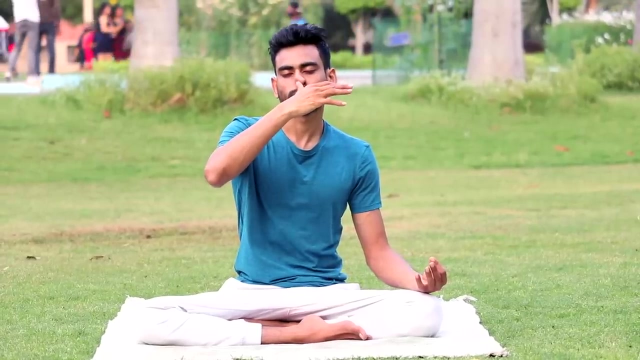 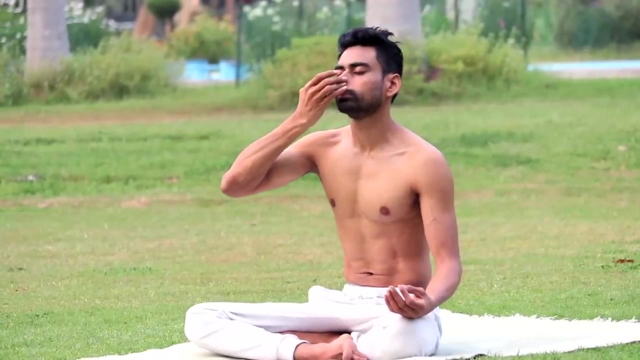 Be mindful of it Throughout. keep a mild focus in between your eyebrows. This is where the Agna Chakra is located. Anulom Vilom is considered Tri Dosh Nashak Pranayama, Which means that it brings in balance between the three basic doshas in our body. 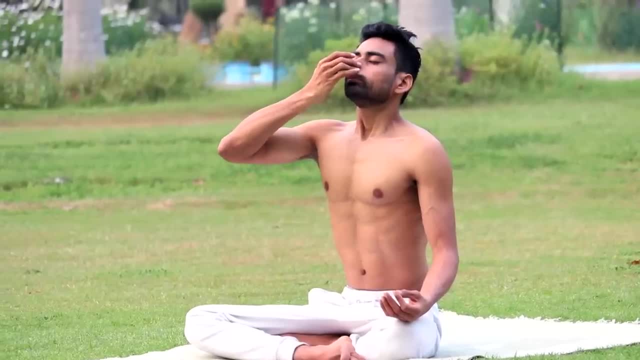 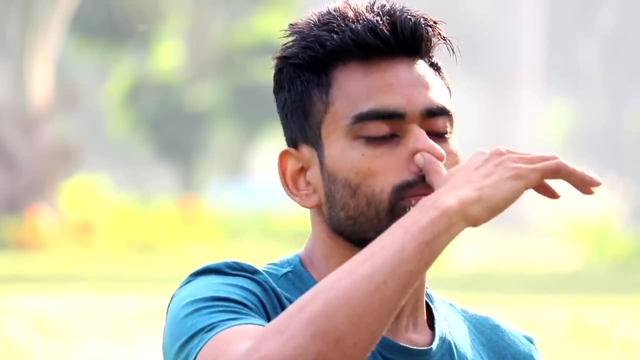 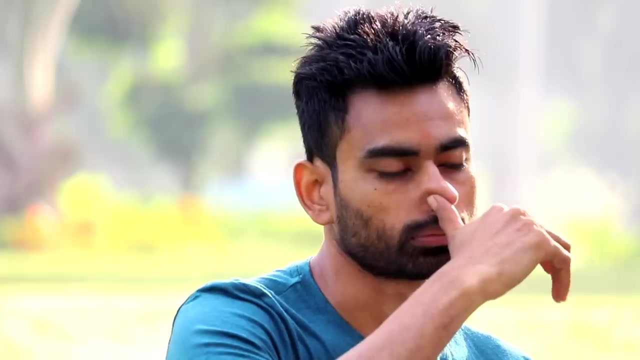 Namely Vata, Pitta and Kapha. So no matter what your body type is, Anulom Vilom will bring about an ideal balance within Our mind has a tendency to keep regretting or glorifying the past and getting anxious. 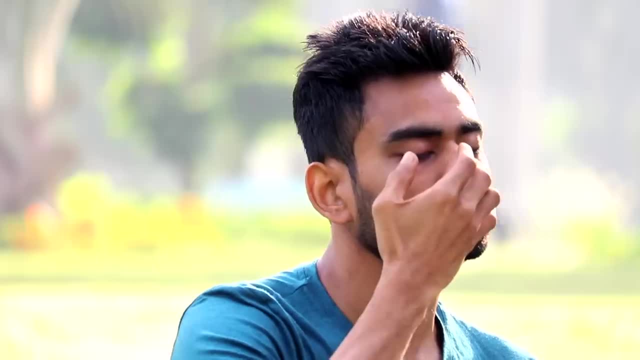 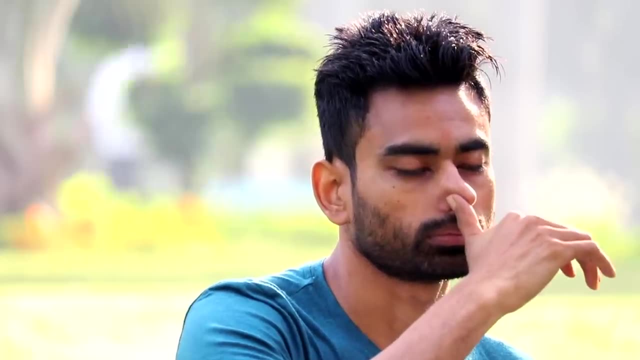 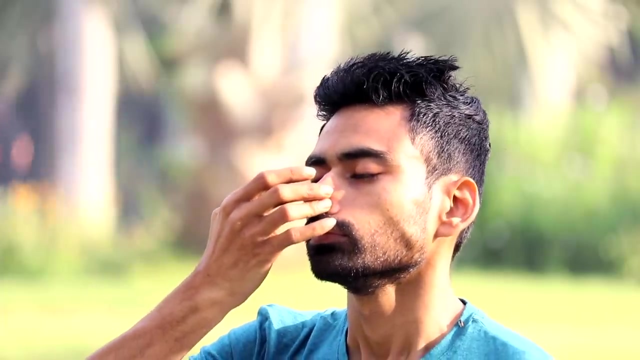 about the future. Nadi Shodan Pranayama Brings the mind back to the present moment. There is a profound reason as to why it is done the way it is done, Why we first inhale from the left nostril. 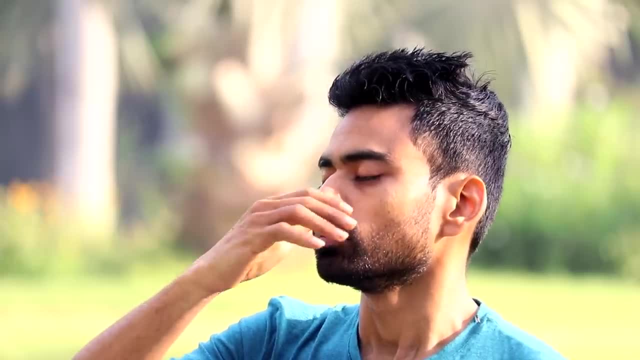 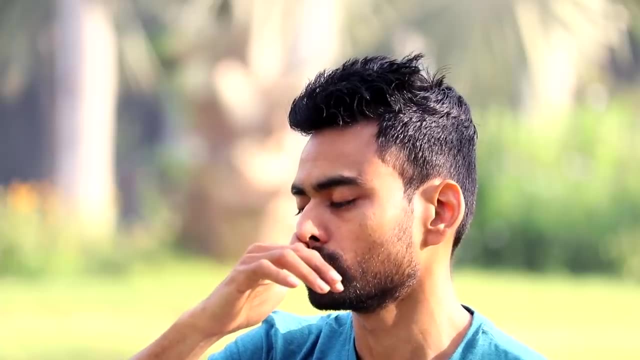 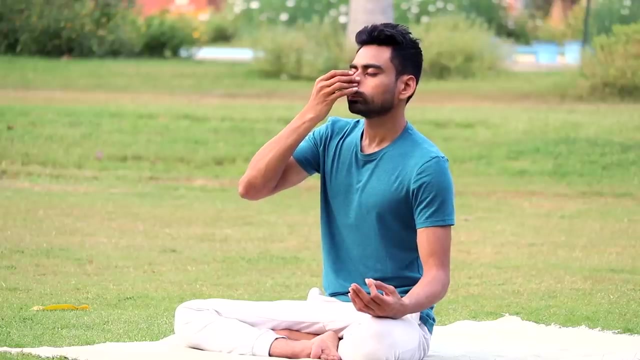 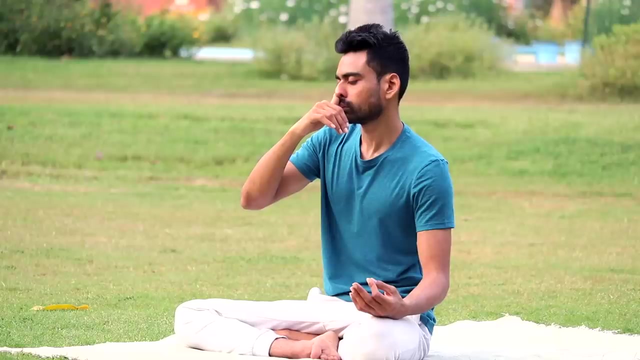 Why only the thumb is placed? Why the middle two fingers are used? To put it simply, it is to bring a balance between the five elements of which our gross body is made of. It clears the energy channels, Ensuring free flow of Prana to every organ of the body. 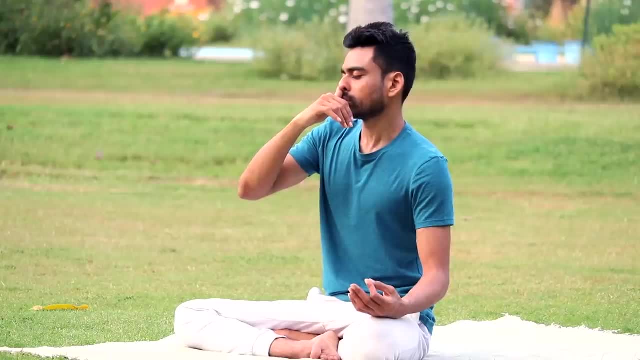 Anulom, vilom is advanced, yet so easy to practice. Do it with that sense of gratitude, with a feeling that you have been given a chance to get connected to your inner self, To unwind the przest89h of your life. 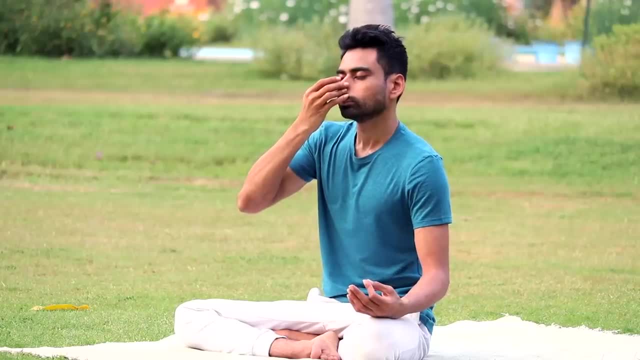 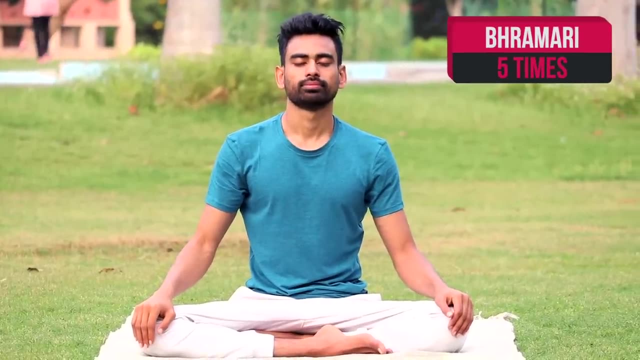 The power of Sanatana Pranayama appeared two ideos earlier in the life On working energy. Prana, Pranayama, Pranayama. it immediately put간 Kelvin Ura, Cross yourself your true nature. Moving on to the last practice of this yoga session: Brahmri or the B-Breath. 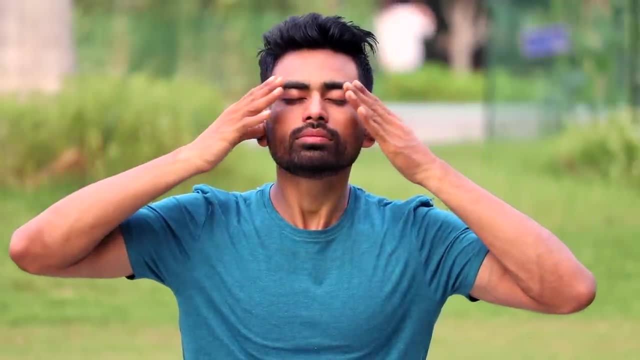 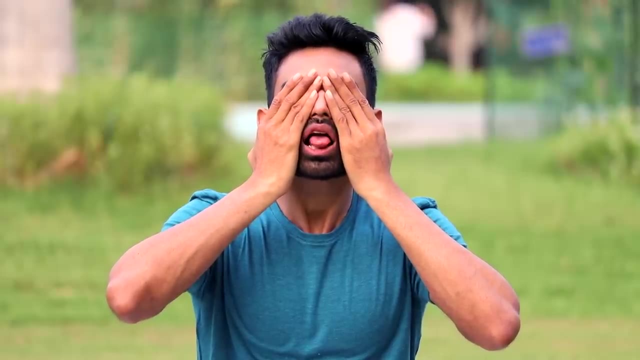 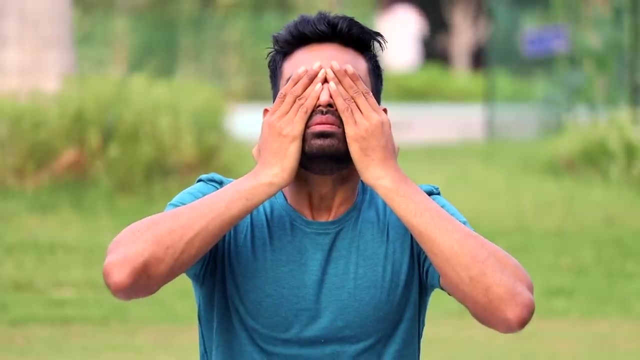 Thumbs closing the ears, index fingers just above your eyebrows and the rest of your fingers softly placed over your eyes. Touch the tip of your tongue to the palate mouth closed. Concentrate in between your eyebrows. Take a long, deep breath through your nostrils and breathe out, making a humming sound of. 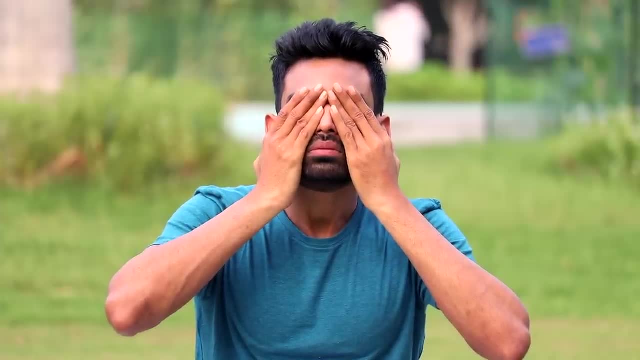 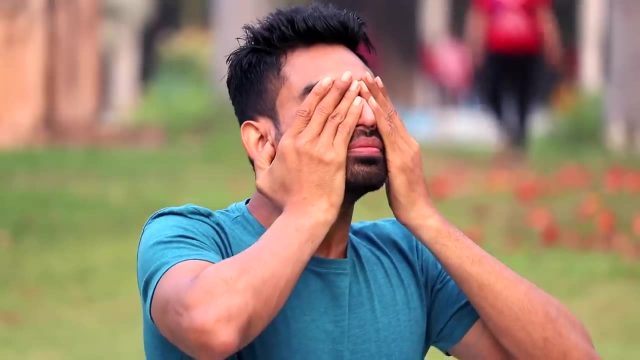 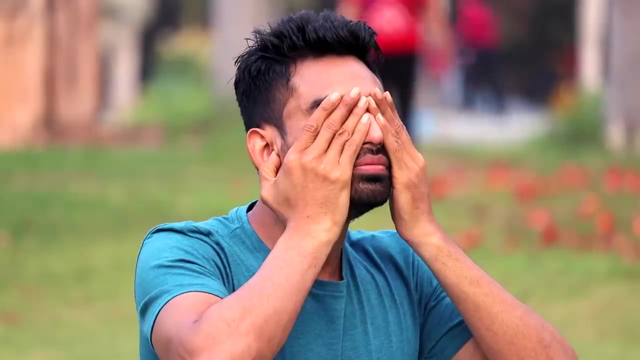 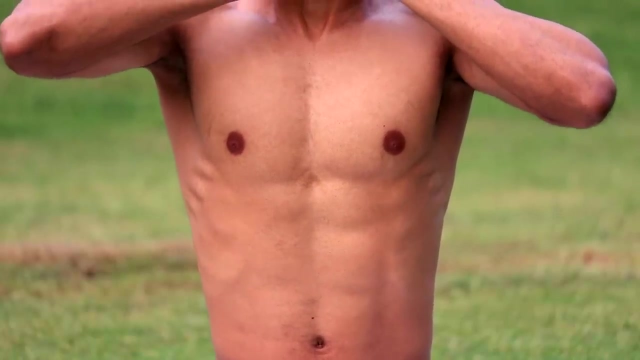 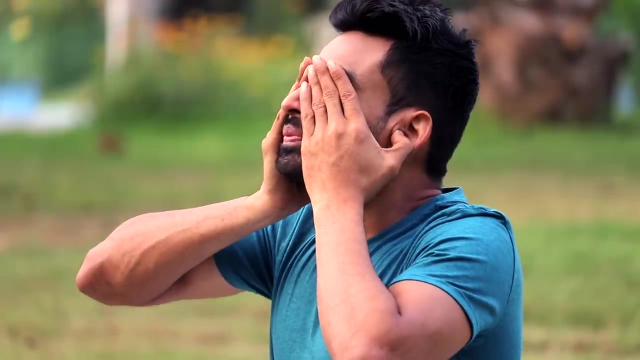 OM. Do it five times. Keep your eyes closed and look through your third eye: the vast emptiness. Assume that you are sitting on the axis and this universe is revolving around you. Visualize that all the positive energies are getting emanated from your body in the 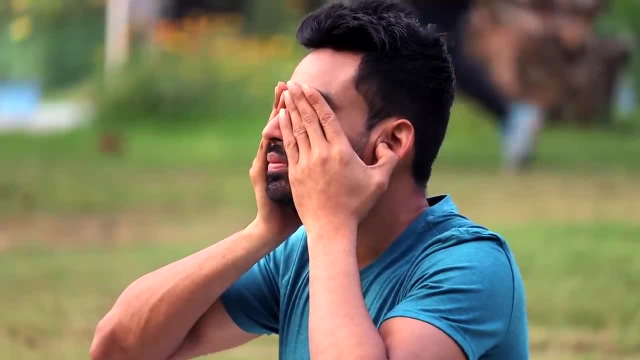 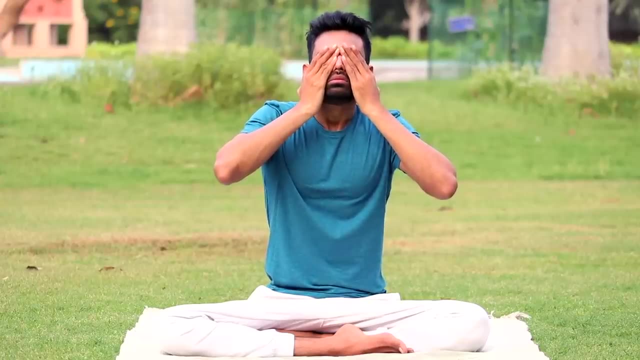 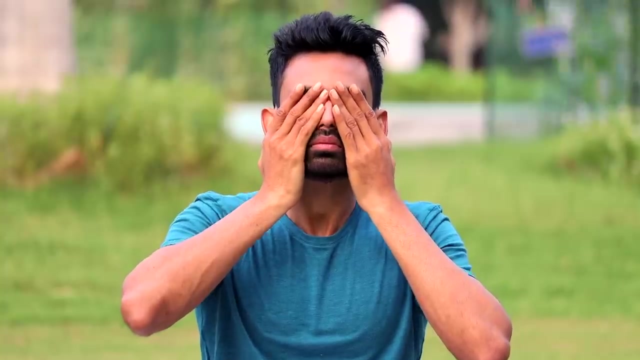 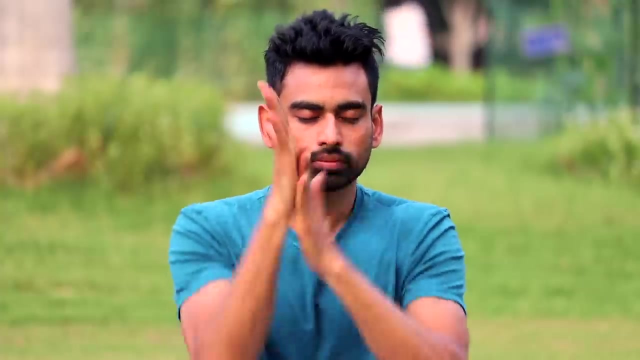 form of humming sound of the bee Stimulating the pineal and pituitary glands. it is a panacea for all problems related to the brain. Now, before opening the eyes, Bring your palms together and rub them vigorously and continuously for a few seconds, and then. 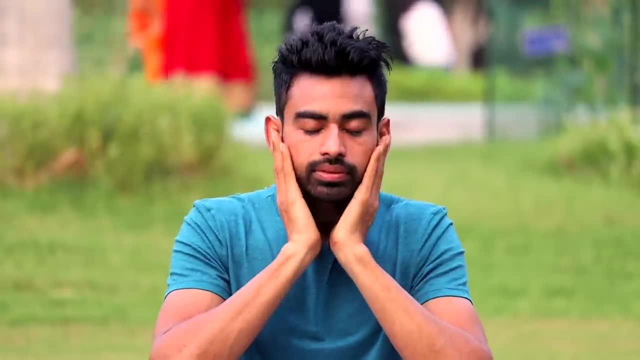 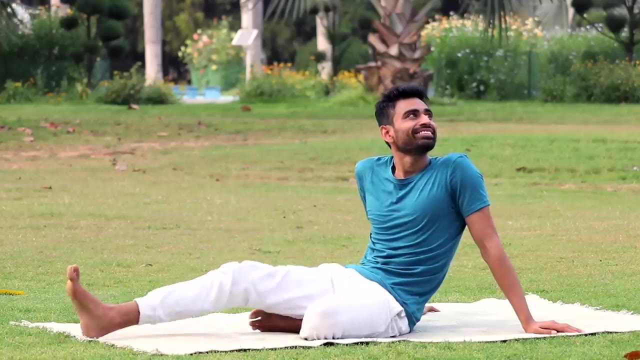 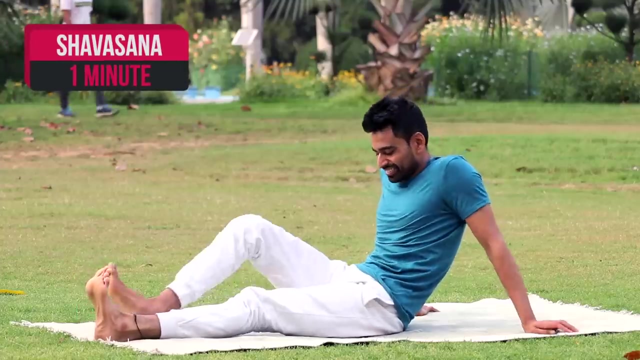 place them on your eyes and face Now slowly open your eyes. peace, calm, serenity- that's what your body is emanating. Now lie down flat on the mat in Shavasana for a minute. It's like a yogic cool down. 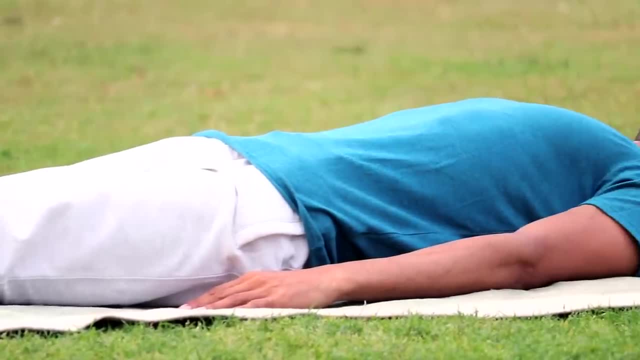 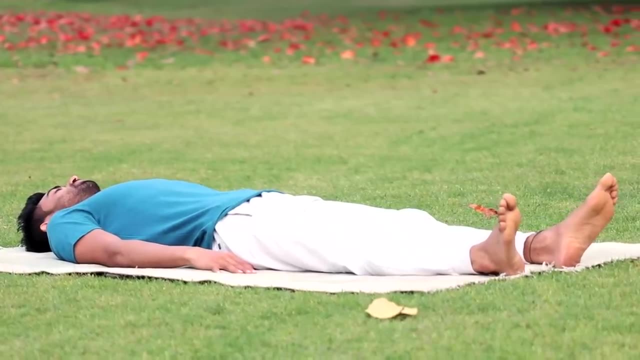 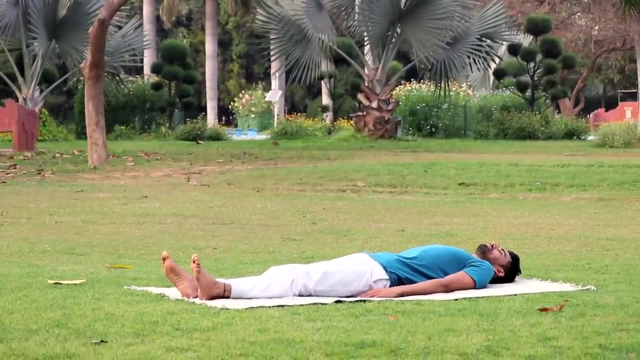 Each cell in your body is grateful to you for completing this session. Every organ in your body is elated. They are delighted, satisfied for being taken care of. Be proud of yourself, Be joyful, You have done it. Thank the universe. 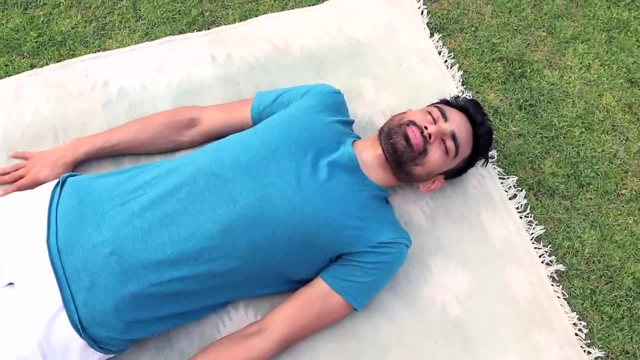 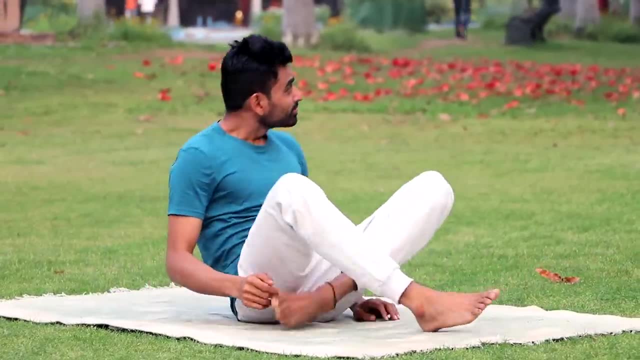 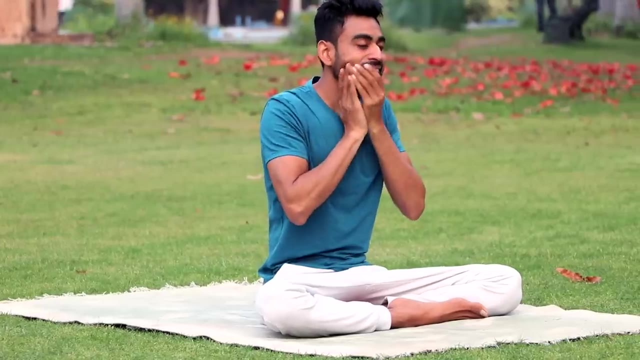 Promise yourself that you will remain cheerful all day long. Promise that you will be polite to others. Promise that you will treat everyone with love and respect. Promise that, no matter what life throws at you, you will take it with a taste of your calmness. 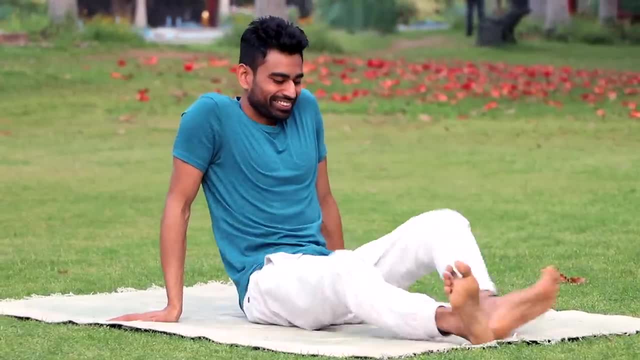 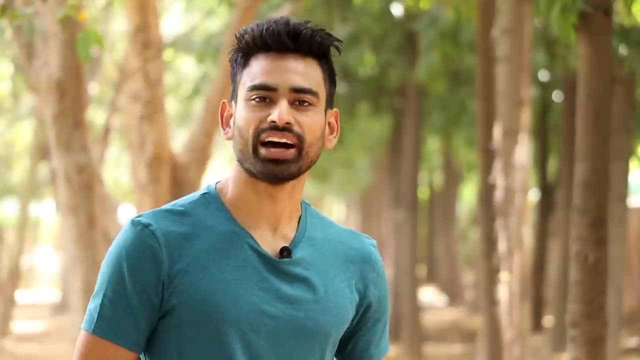 Well done. You have completed this yoga session. I bow down to the divine in you. I'll see you tomorrow again, Namaste. So, friends, how was it? I hope you enjoyed this yoga session. Feel free to take breaks in between. 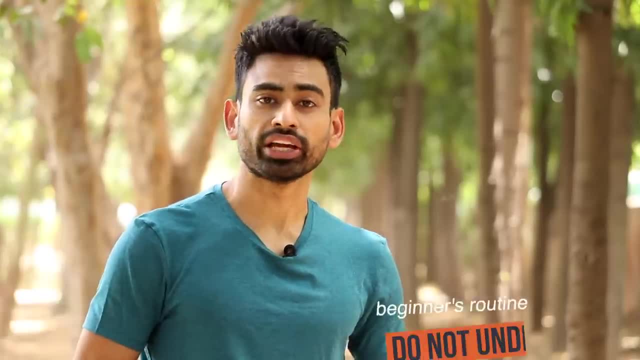 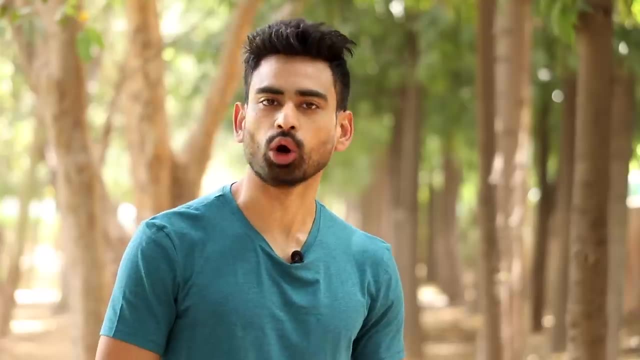 Yoga is all about being comfortable and calm. This is a beginner's routine, But do not underestimate the benefits that you can reap from it. Trust me, this 30 minutes daily yoga will take you a long way. You will thank yourself for the priceless happiness, calmness and health that you will. 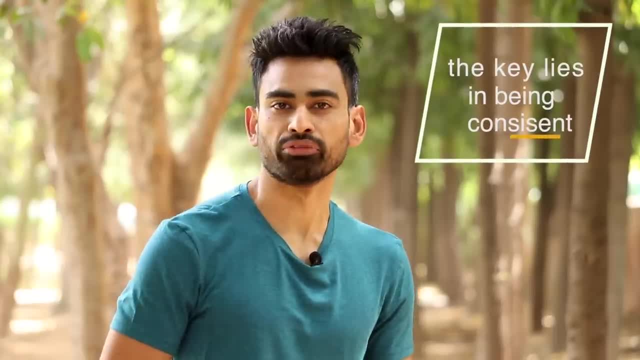 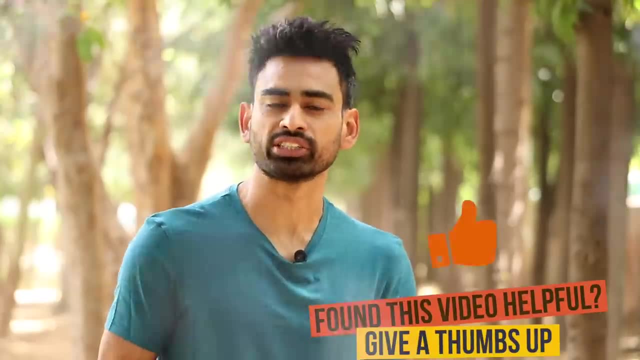 obtain from it. One week is good enough to experience the benefits. However, the key lies in being consistent. If you found this yoga session helpful and would want me to make more such sessions, please give it a big thumbs up. If you are looking for a genuine, toxin-free face wash, Mama Earth's Uptan Face Wash is 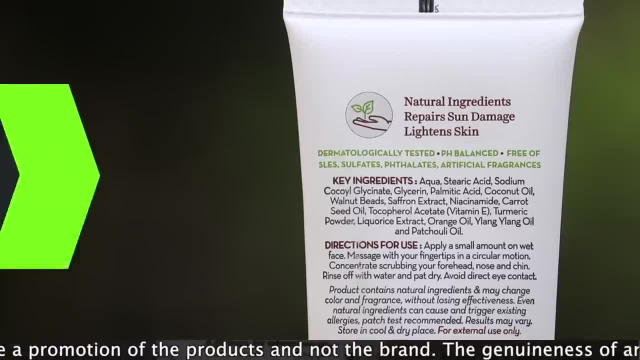 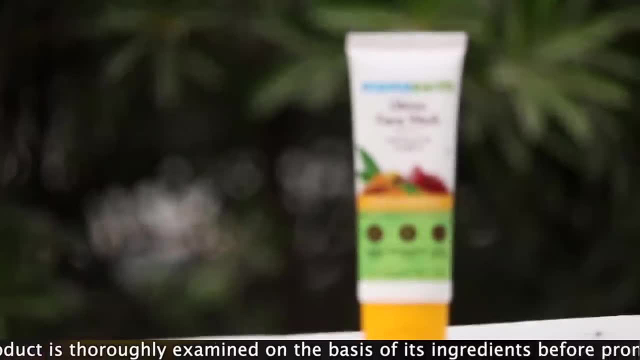 one good option in the Indian market. Go through its ingredients and you will find that it has no sulfates, parabens, EDTAs or other harsh chemicals added in it. Rather, it is made from safe chemicals, along with herbal extracts of turmeric saffron. 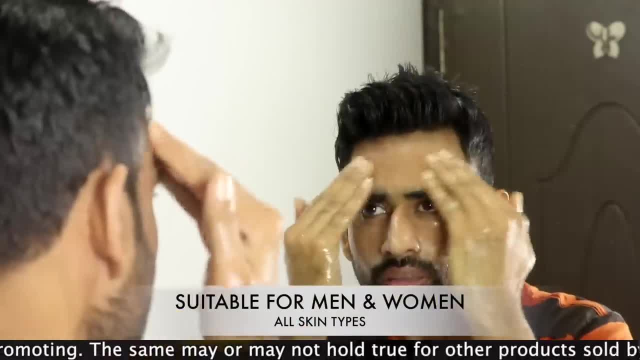 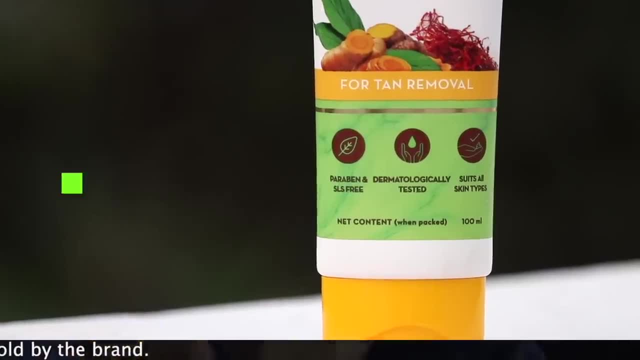 and various skin-friendly essential oils. Mama Earth's This Tan Removal- Uptan Face Wash is suitable for all skin types and can be used by both men and women. Mama Earth's This product is dermatologically tested and is made in India. To buy it, click on the link down in the description box. 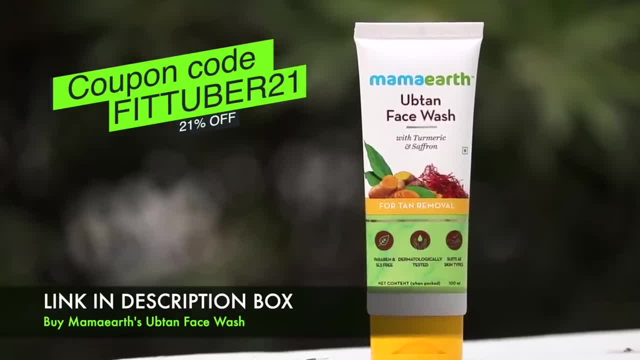 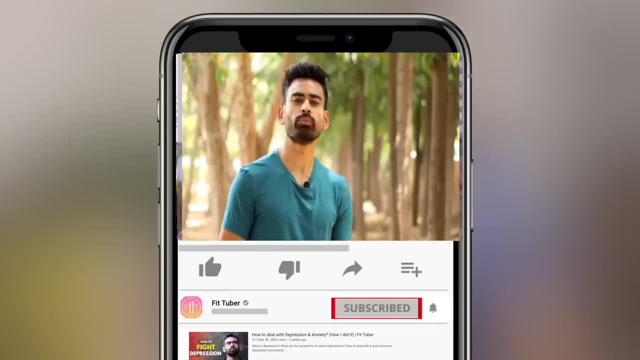 Do not forget to apply the special discount coupon to get 21% off on your order. So, friends, that's all for this video. You can now support my work by clicking on the join button below. Please do remember to subscribe to my channel. hit that bell icon so that you never miss. 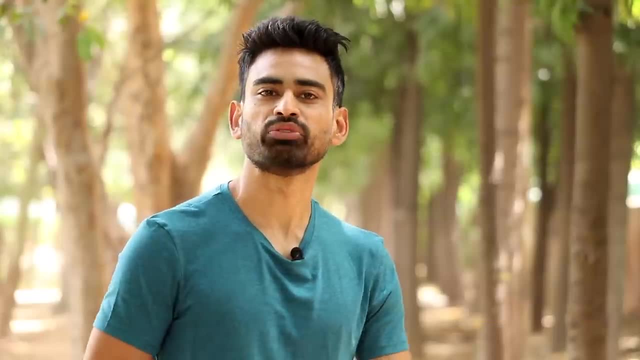 a video from me. You can also follow me on Instagram. My name is Vivek. I thank you so much for watching.